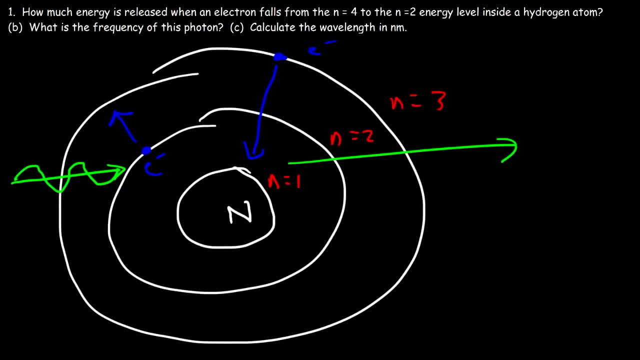 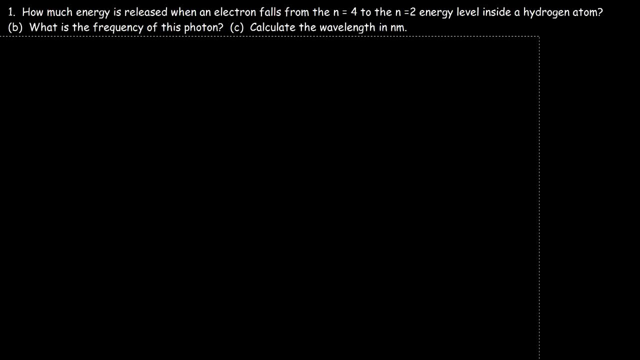 or absorbed when an electron moves from one energy level to another. So let's read the first question: How much energy is released when an electron falls from the n equal 4 to the n equal 2 energy level inside a hydrogen atom? Now the 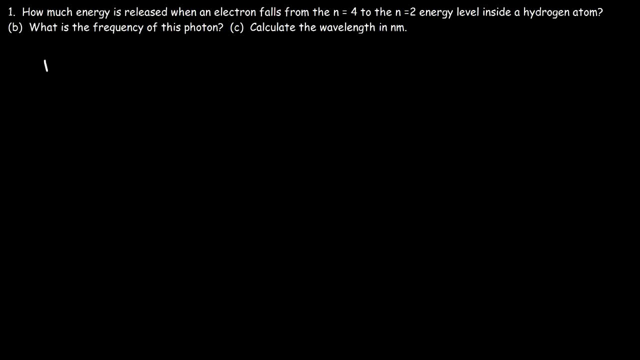 equation that you need to calculate. it is this equation: E is equal to negative, 2.178.. times 10 to the minus 18 joules, multiplied by 1 over n final squared, minus 1 over n initial squared: N initial is the original energy level, which is the 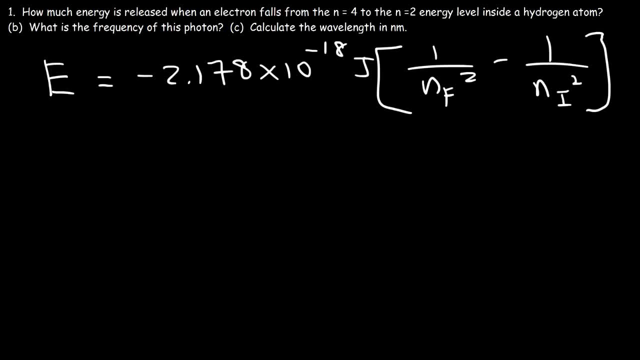 fourth energy level, N final, is where the electron is going to. That is the second energy level. So all we need to do is plug those numbers into the equation. We can find out how much energy is released from an electron within a hydrogen atom. So let's go ahead and do that. 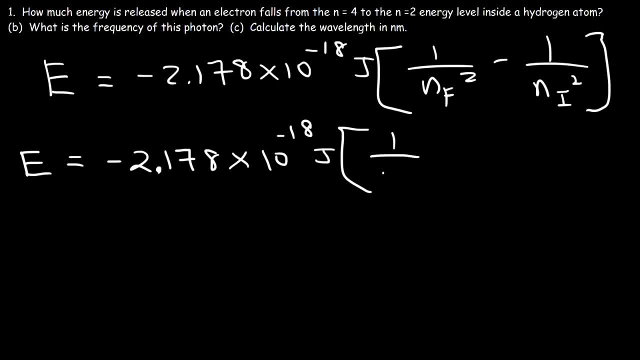 So n final in this problem is 2.- Don't forget to square it- And n initial is 4.. So 1 over 2 squared, 2 squared is 4 and 4 squared is 16.. So we got 1 fourth minus. 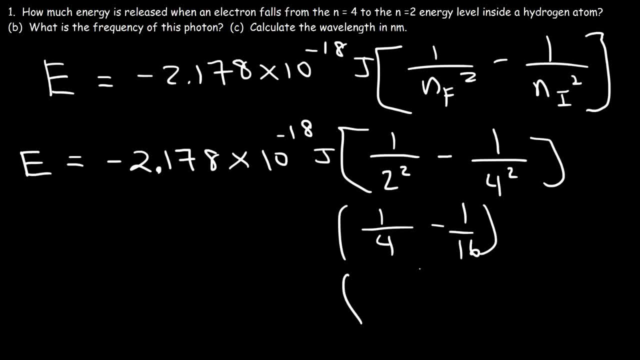 1 over 16.. And that's equal to 3 over 16, which is, as a decimal, .1875.. So let's go ahead and multiply these two numbers, So you should get negative 4.084 times 10 to the negative 19 joules. 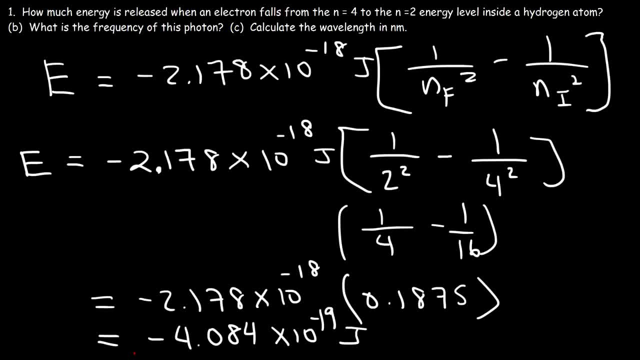 So that's the number you need to get. So that's how much energy is released when an electron falls from the fourth to the second energy level? Now here's a question for you. Why is this answer negative? Recall that when it falls from, let's say, a high energy level to a low energy level, 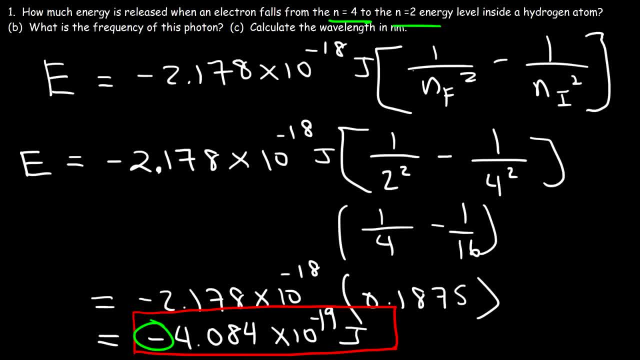 a photon is emitted, so the electron is losing energy, and that's why it's negative. If the electron jumped from, let's say, the second to the fourth, it would be absorbing energy, so E would be positive. So that's why we have a negative sign to show that energy is being released as the 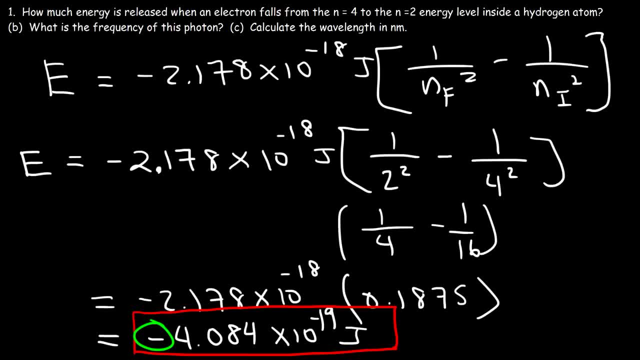 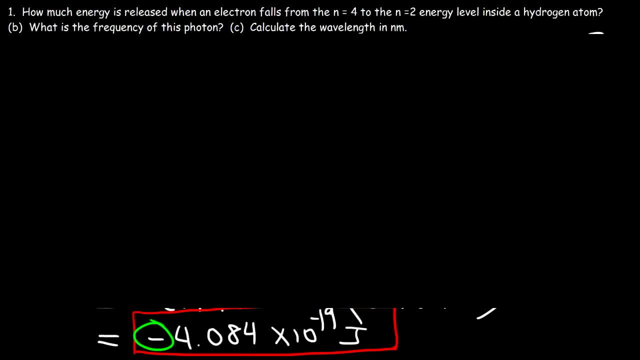 electron falls to a lower energy level. Now let's move on to part. How can we calculate the frequency, now that we have the energy of the photon? Now, if you recall from earlier videos, the energy of a photon is equal to the product. 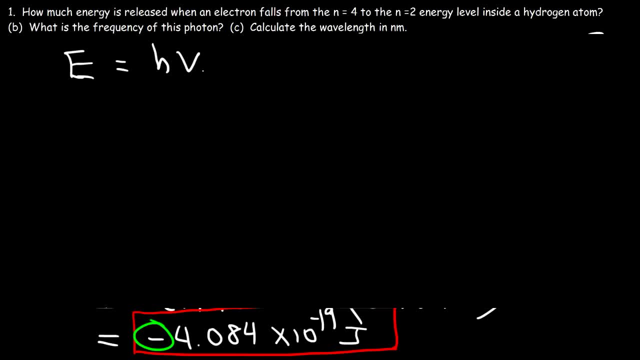 of Planck's constant and the frequency of that photon. So to calculate the frequency it's simply the energy divided by Planck's constant. So it's going to be 4.084 times 10 to the negative 19 joules. 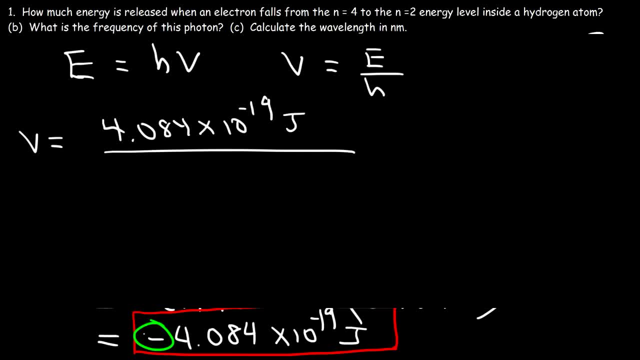 You don't need the negative sign, because frequency is always positive. The purpose of the negative sign is to tell us if a photon is being absorbed or released by an electron. Okay, So let's go ahead and divide those two numbers, So you should get 6.164 times 10 to the 14 hertz, or 1 over seconds. 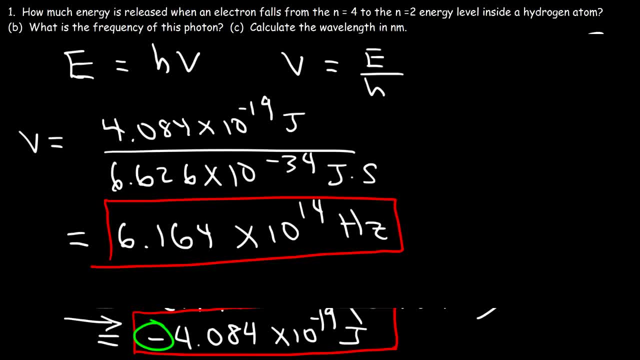 So that's the frequency. Now that we have the frequency, let's move on to part. Let's calculate the wavelength of the photon in nanometers. Now, the speed of light is the product of the wavelength and the frequency. So the wavelength is the speed of light divided by the frequency. 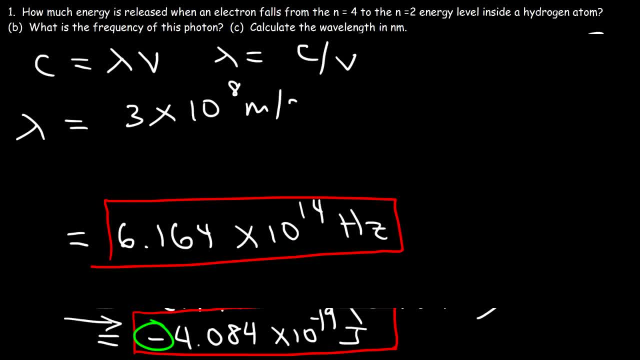 The speed of light is 3 times 10 to the 8 meters per second, and the frequency is 6.164 times 10 to the 14, with units 1 over seconds. Now let's go ahead and put that in the calculator. 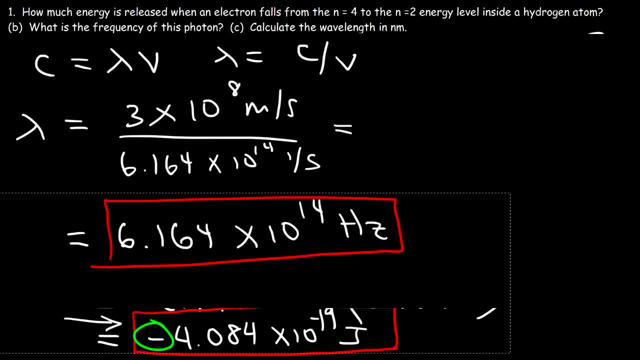 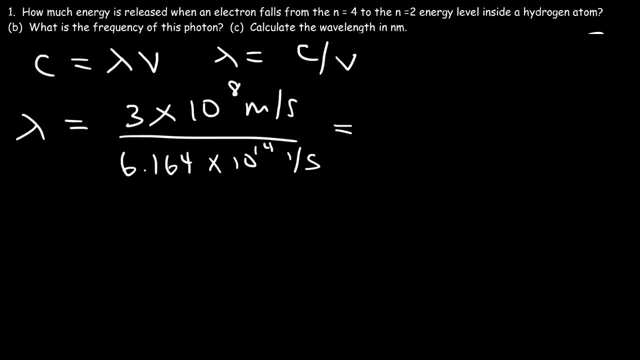 So I got 4.87 times 10 to the negative 7 meters. Now we need to convert this into a�. What I'm going to do is I'm going to convert this into aλ. So that's 4.87 times 10 to the negative 9 meters. 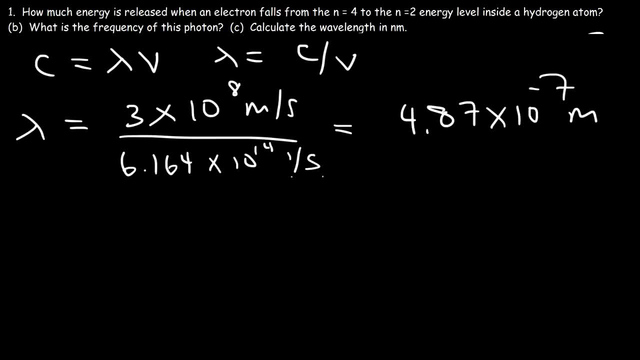 That's 4.8 plus 3.7 plus 2.3.. That's 3.8.. Now the reaction is going to be 2 times 15 volts per second. per second per second per meter to nanometers. So how can we do that? Now, you need to know that 1 nanometer is equivalent to 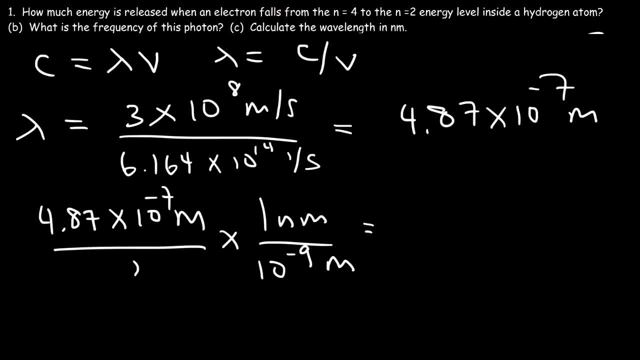 10 to the minus 9 meters. So you can take the answer that we have 4.87 times 10 to the minus 7, and divide it by 1 times 10 to the negative 9.. And so this is equal to 487 nanometers. 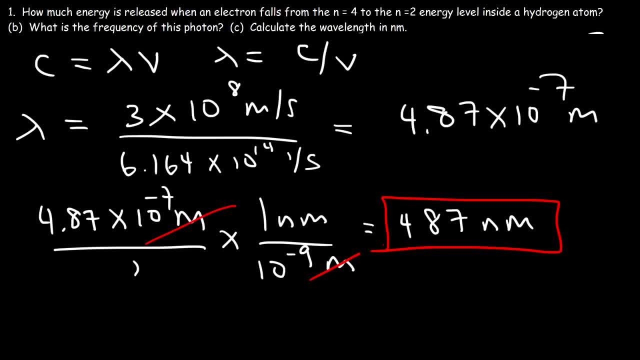 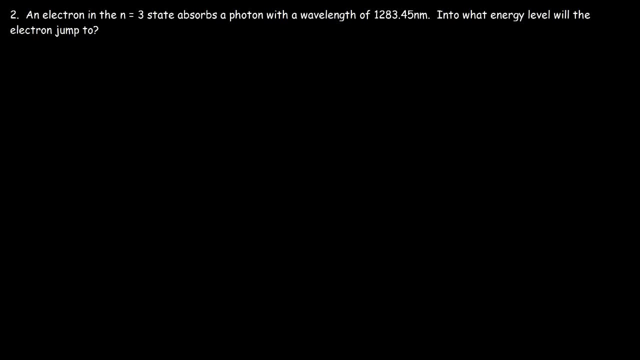 So that's how you can calculate the wavelength of this photon. Number two: an electron in the third energy level, or n equal 3 state, absorbs a photon with a wavelength of 1283.45 nanometers. And so what energy level will the electron jump to? 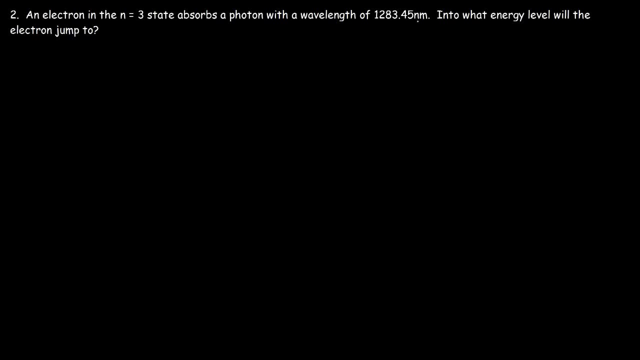 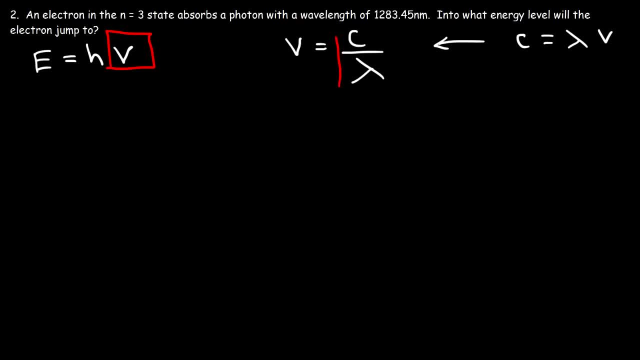 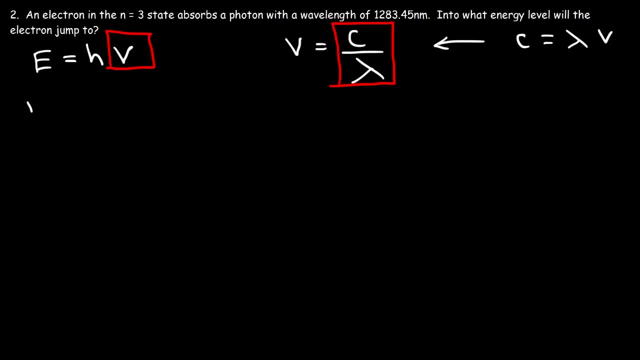 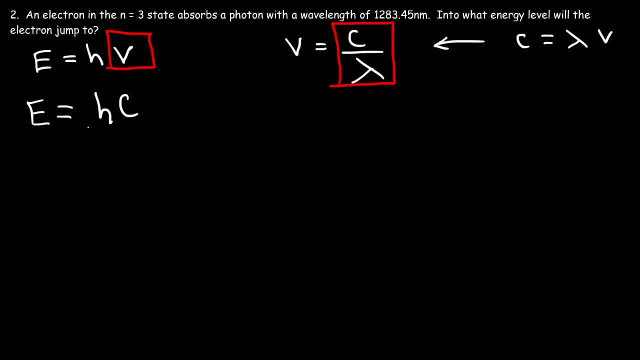 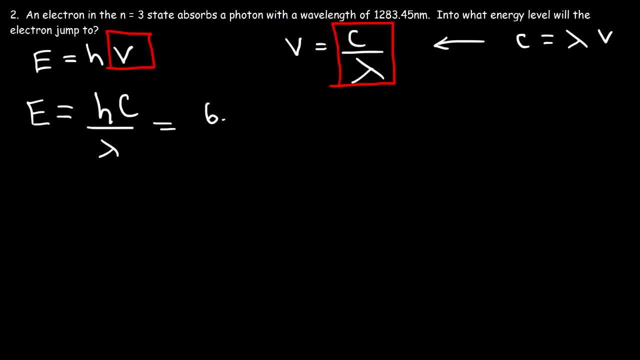 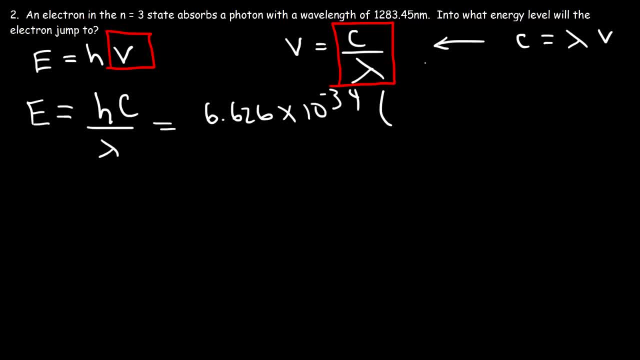 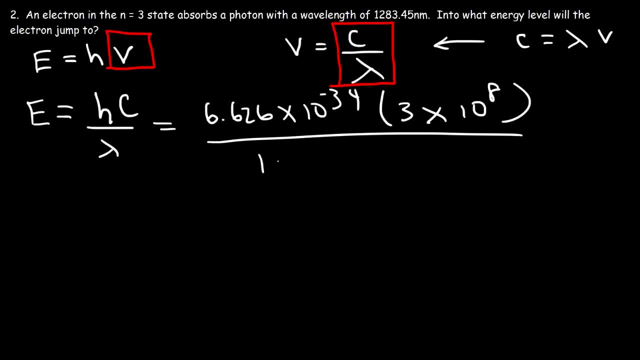 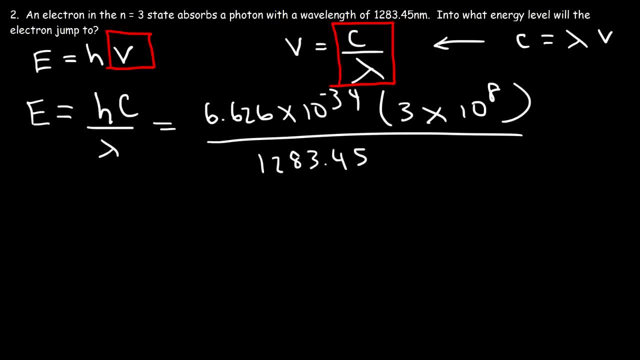 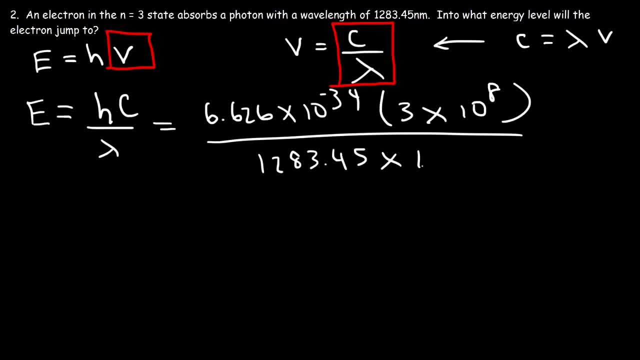 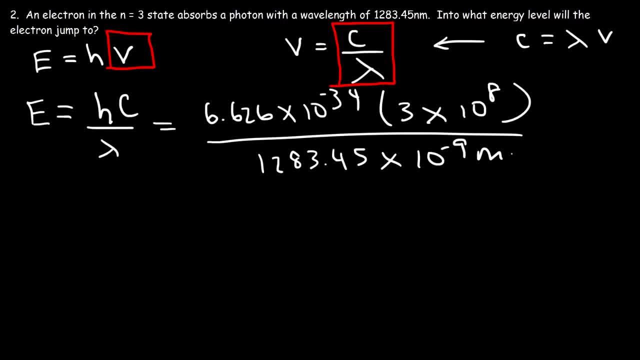 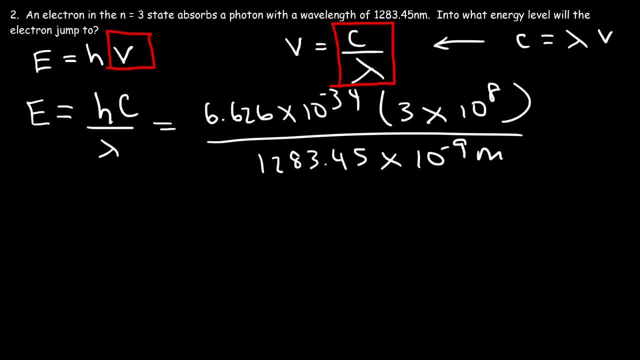 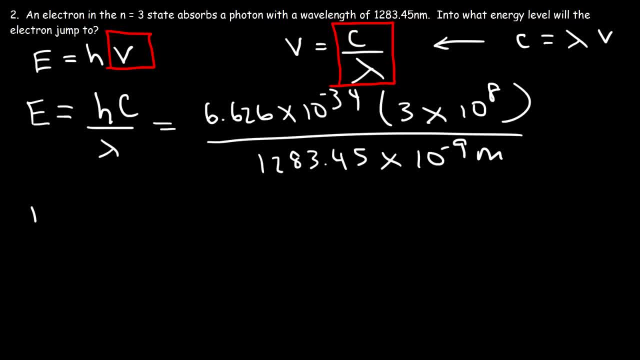 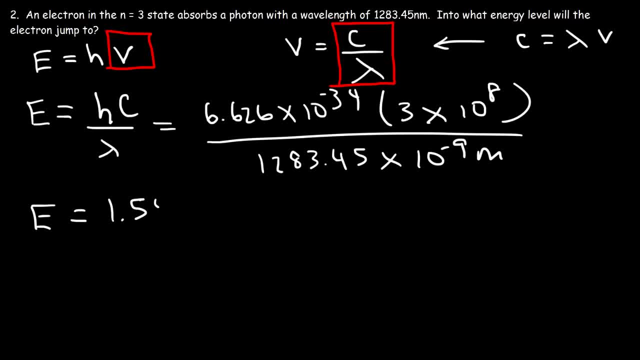 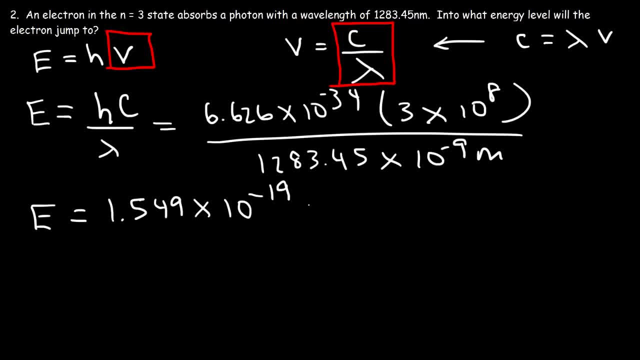 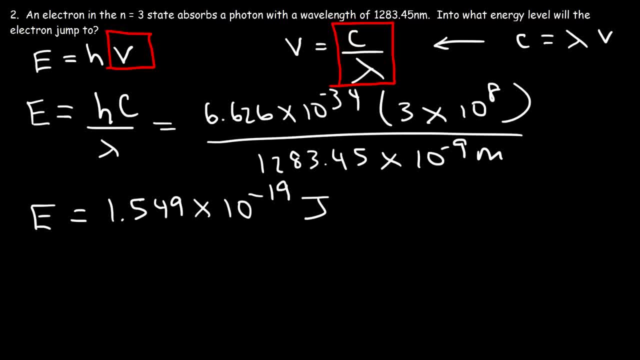 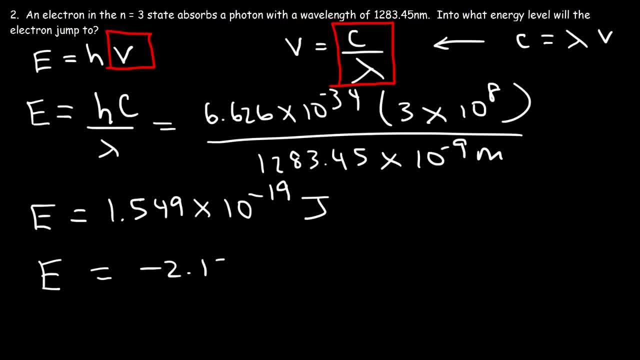 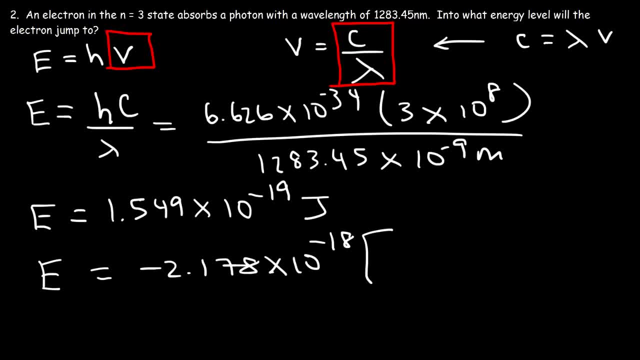 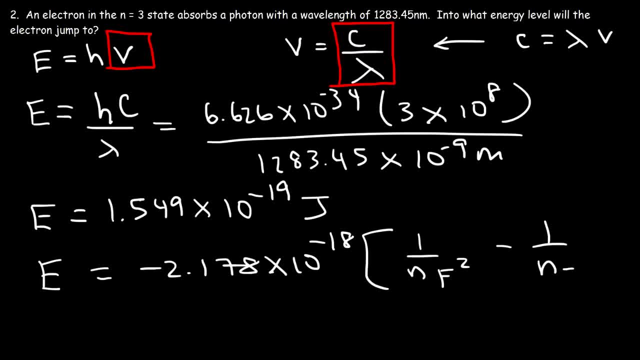 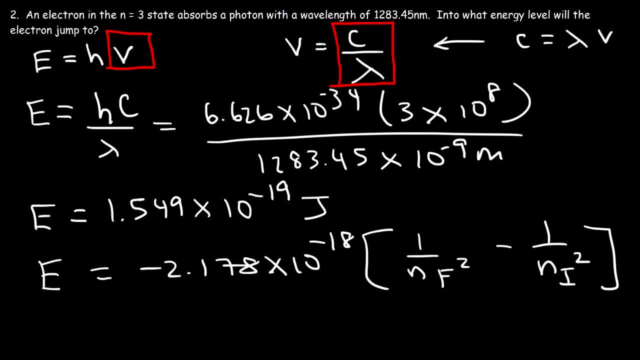 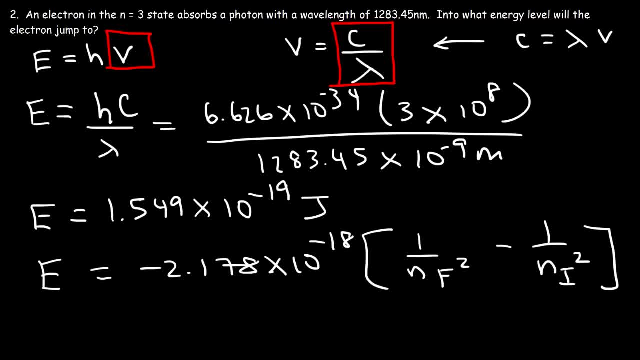 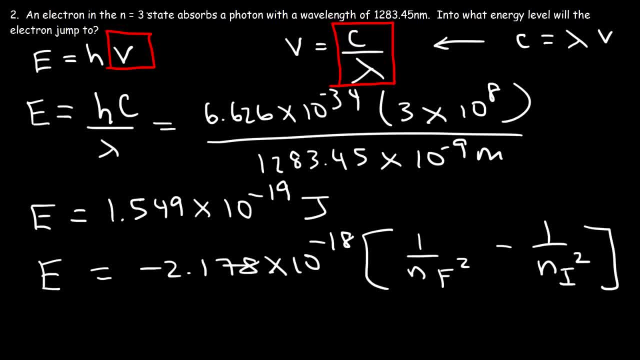 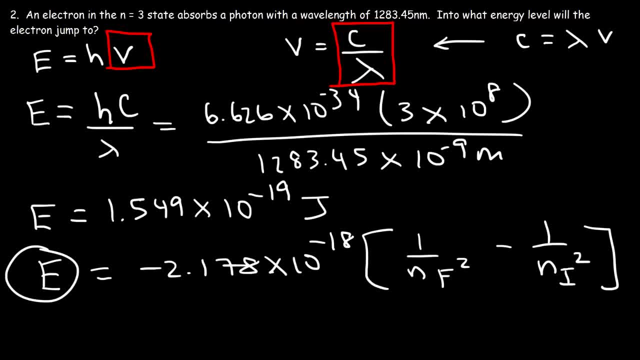 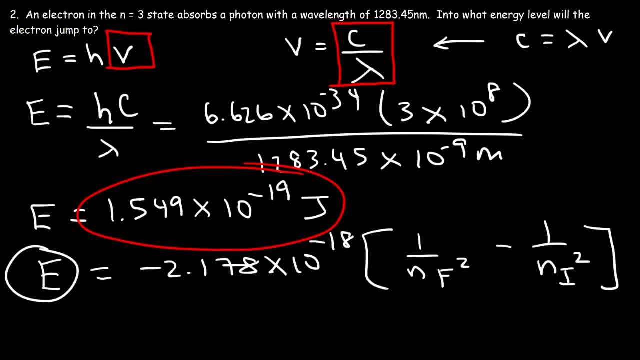 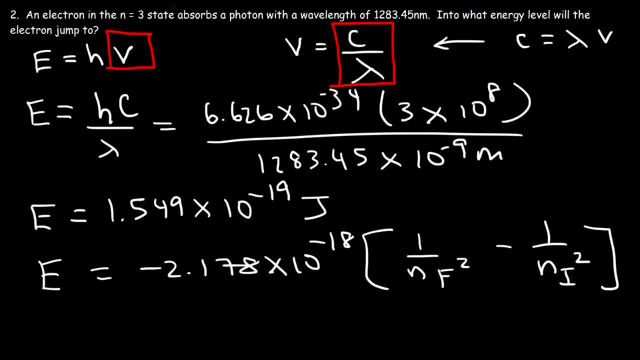 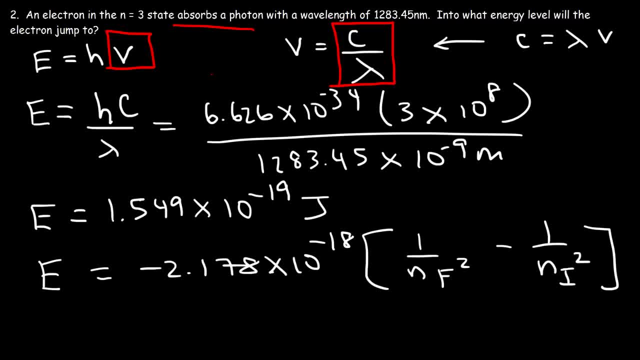 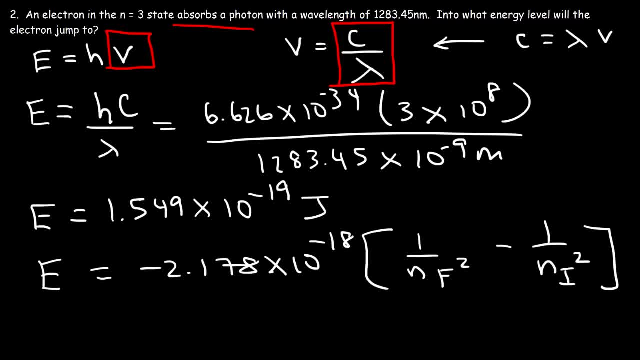 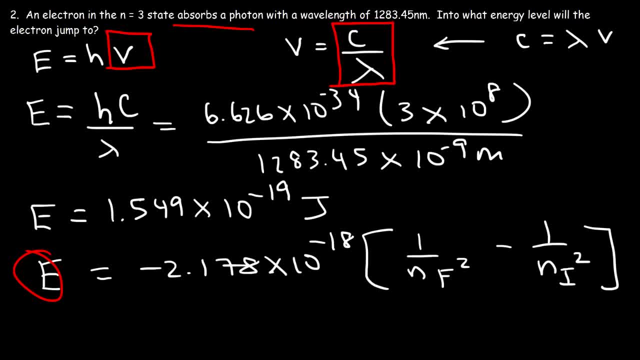 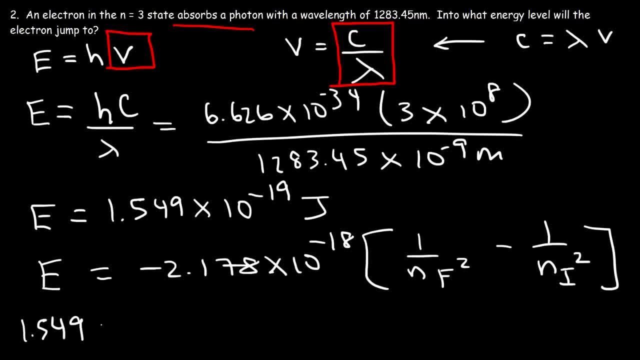 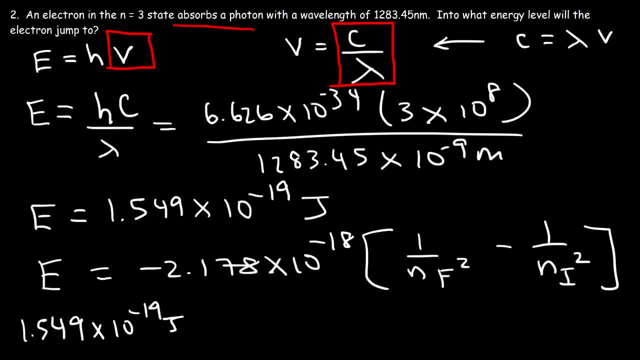 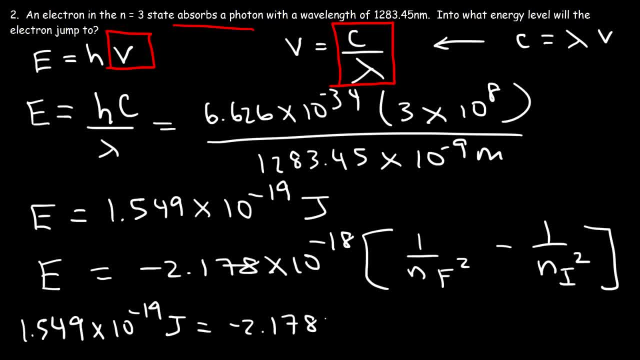 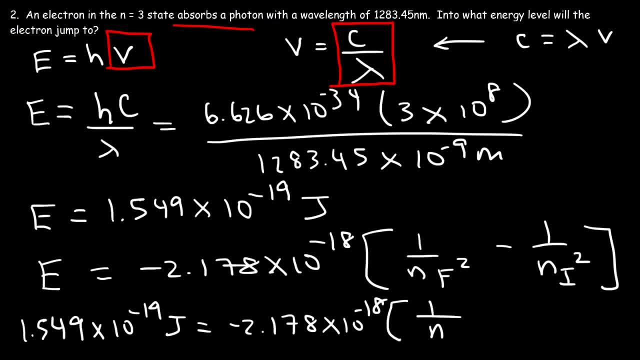 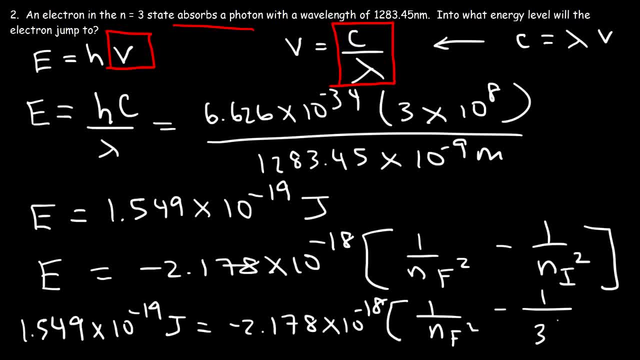 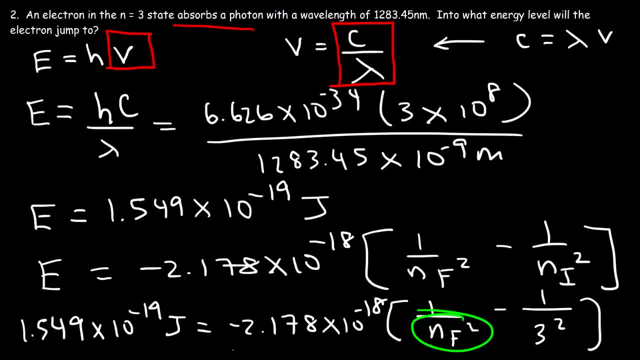 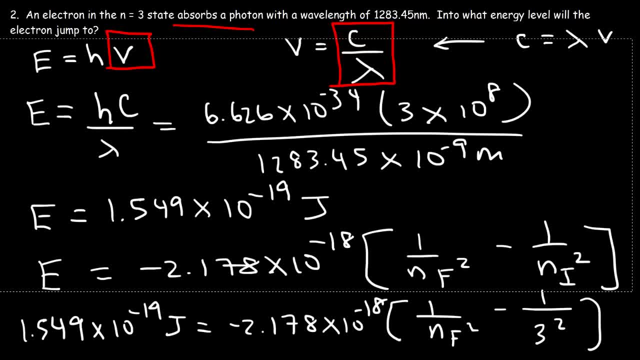 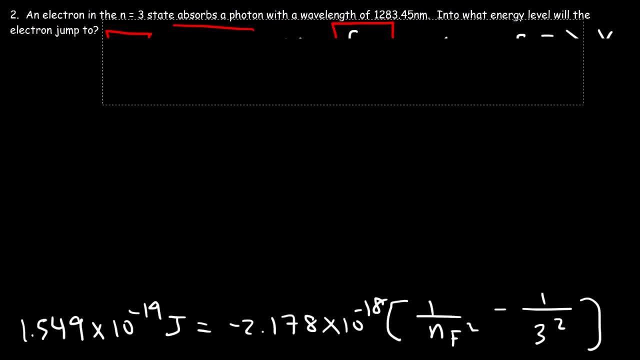 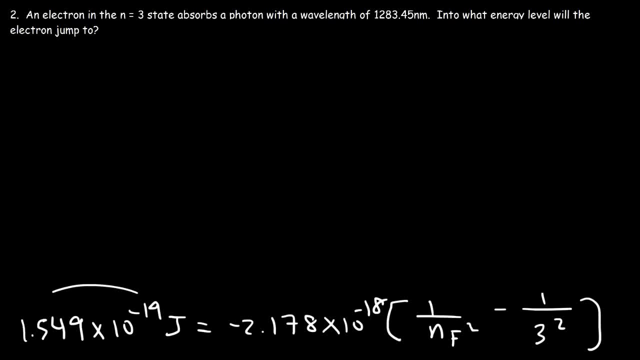 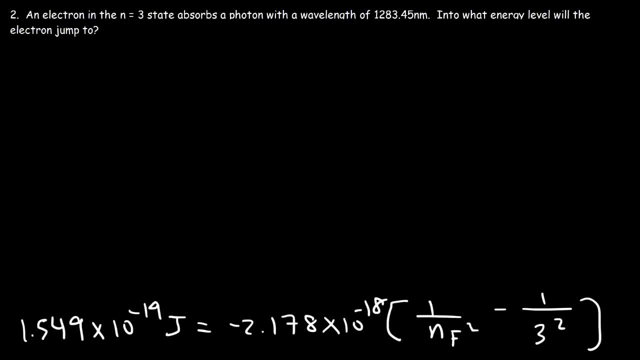 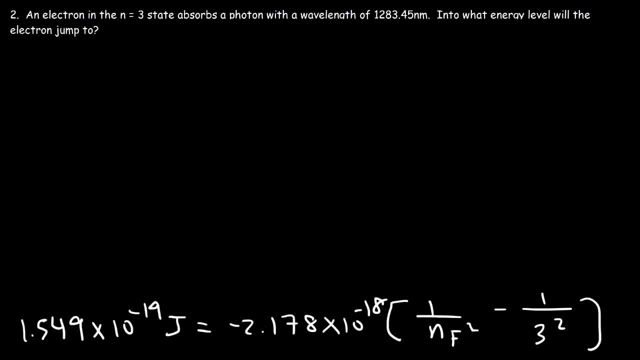 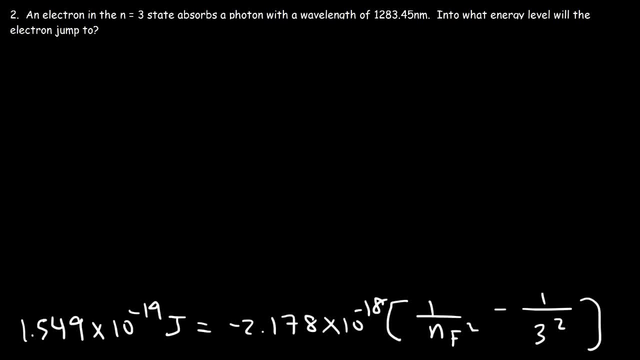 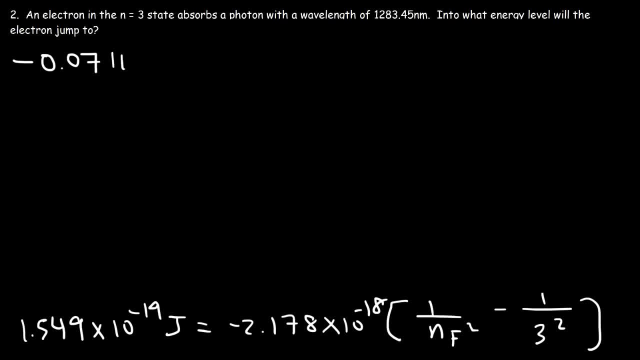 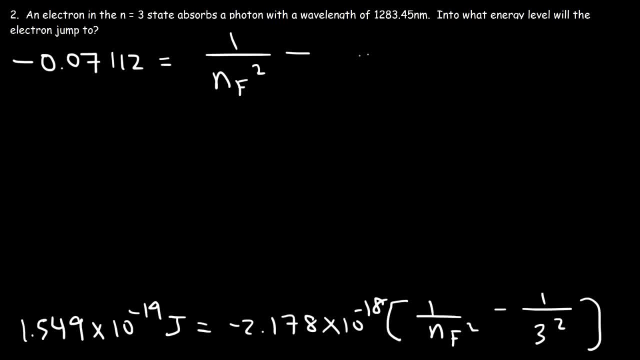 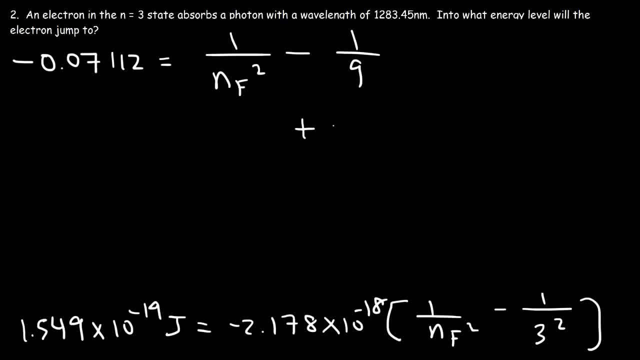 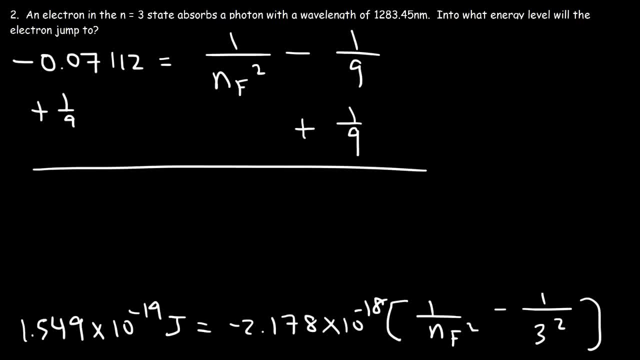 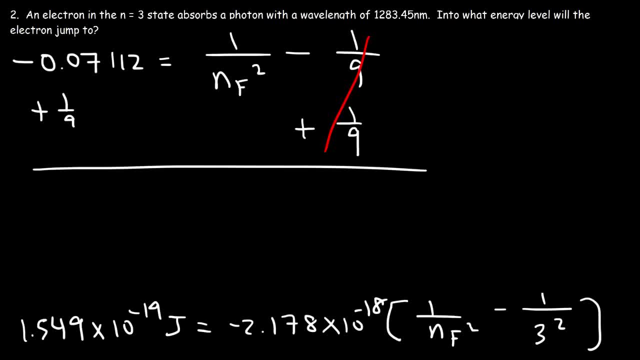 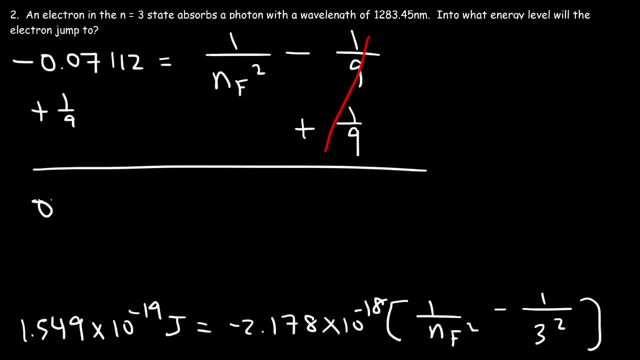 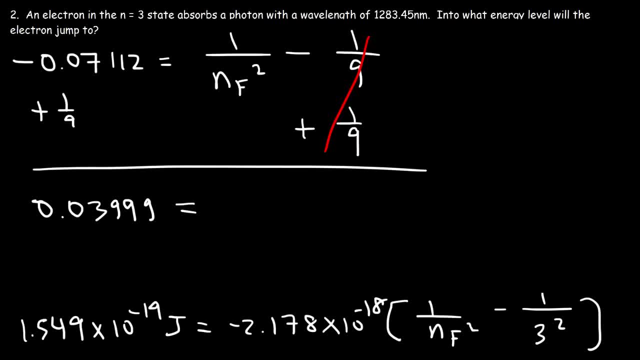 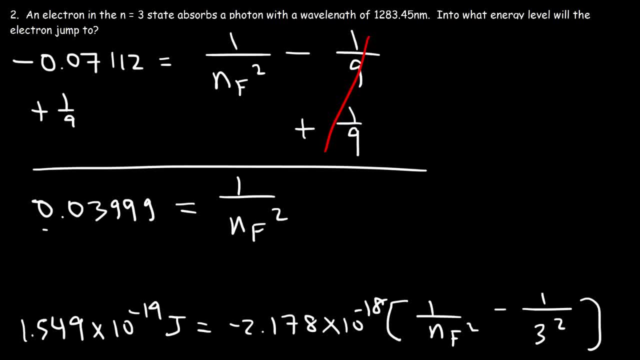 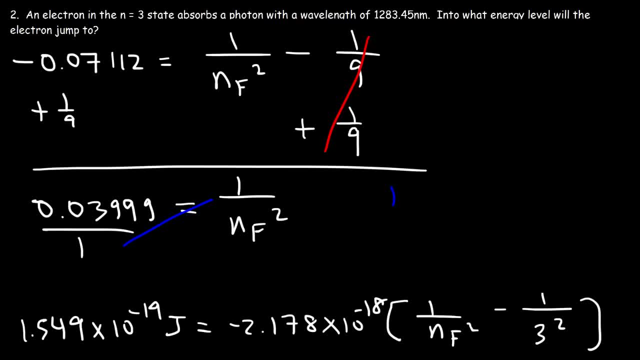 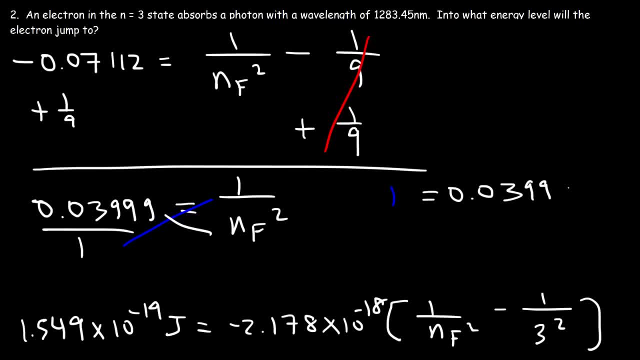 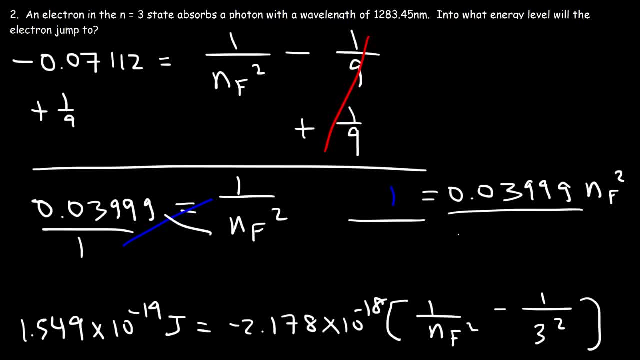 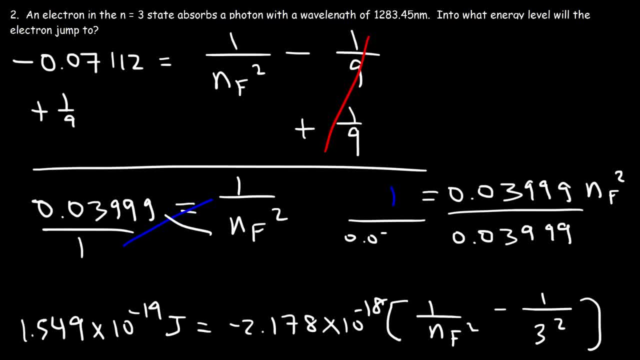 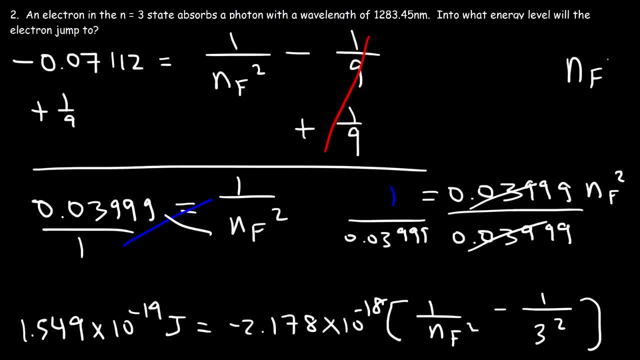 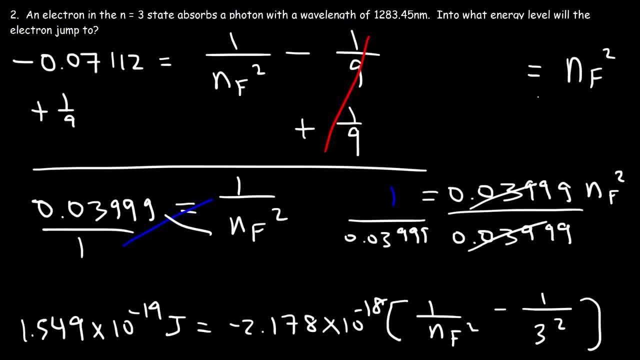 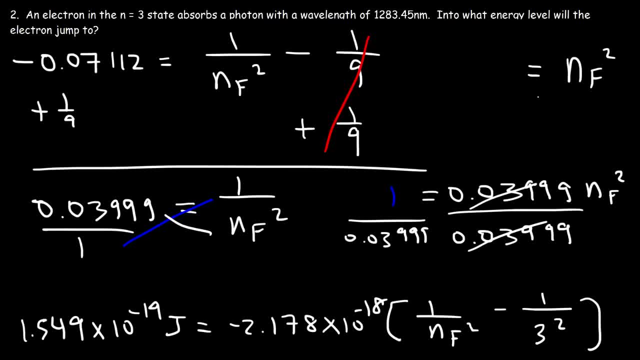 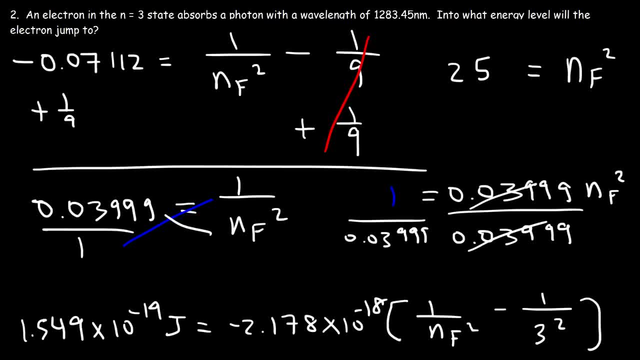 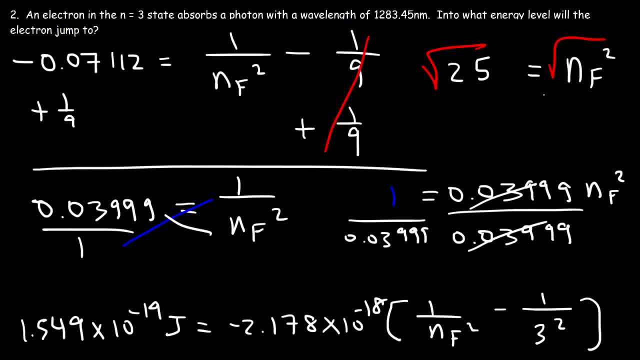 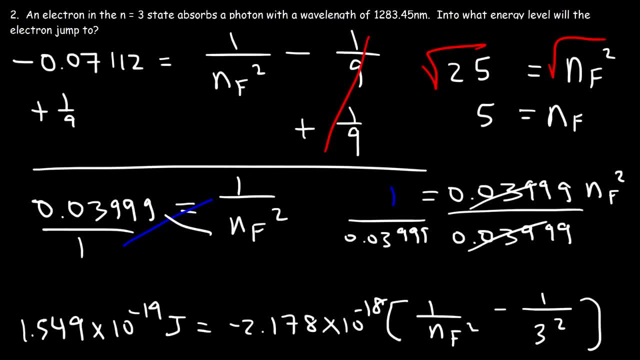 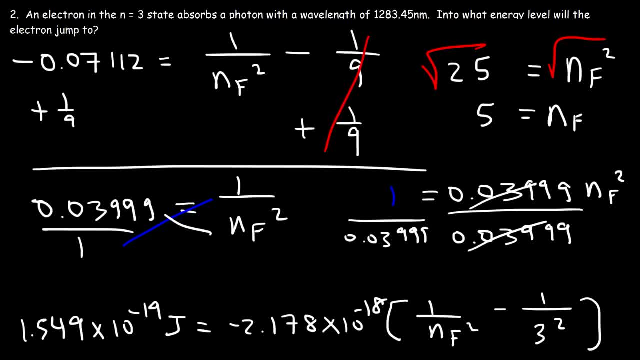 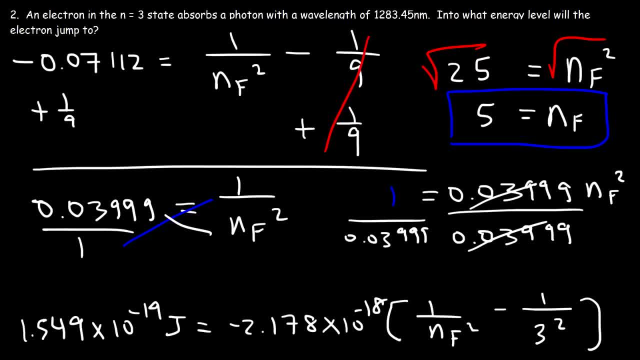 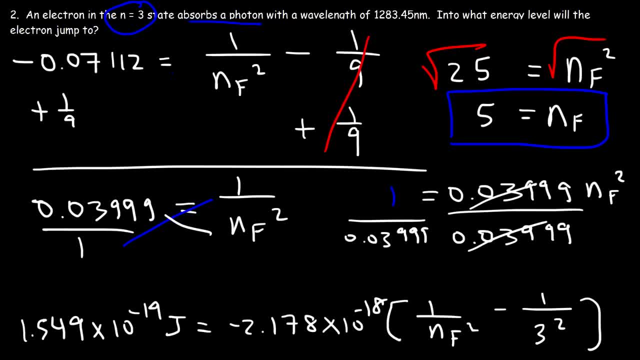 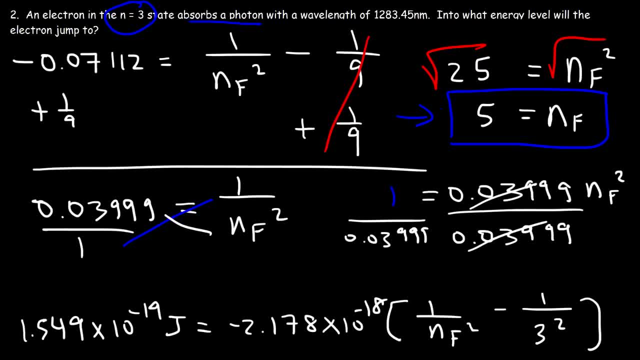 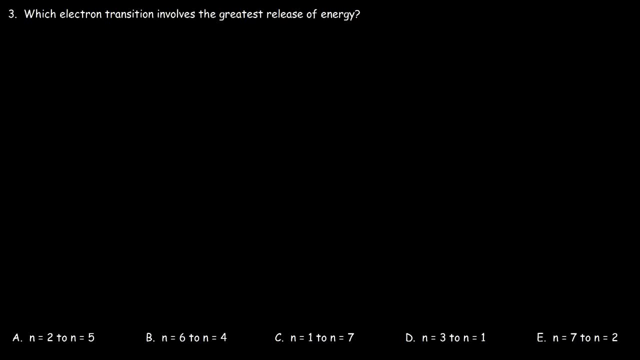 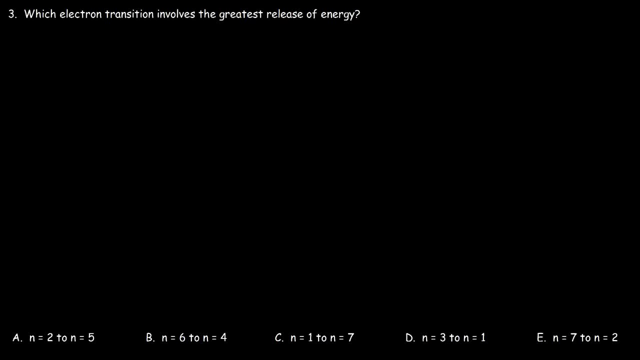 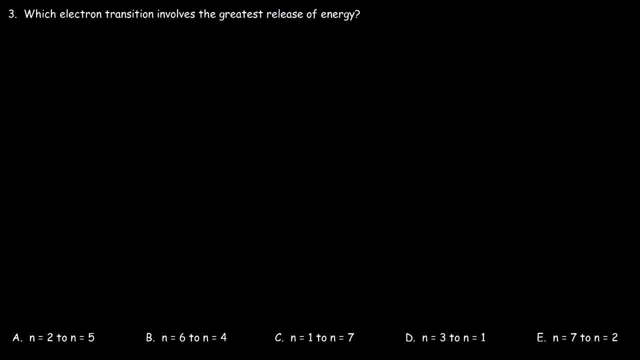 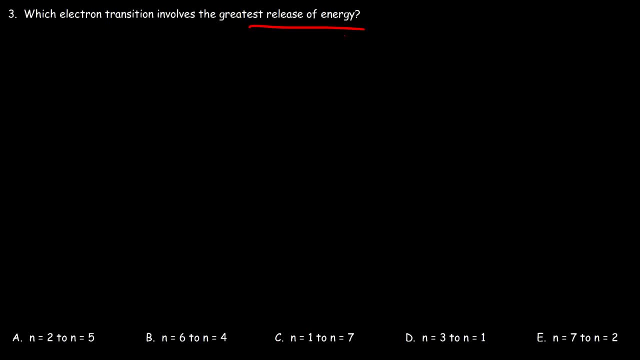 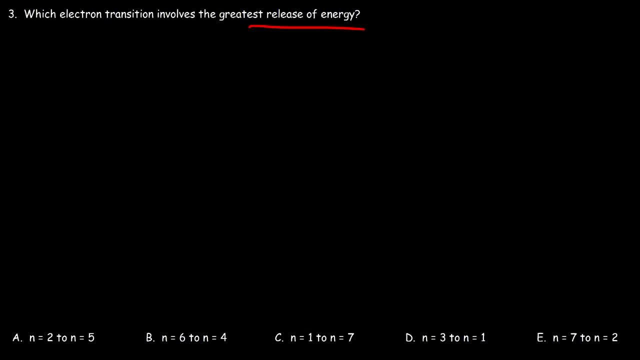 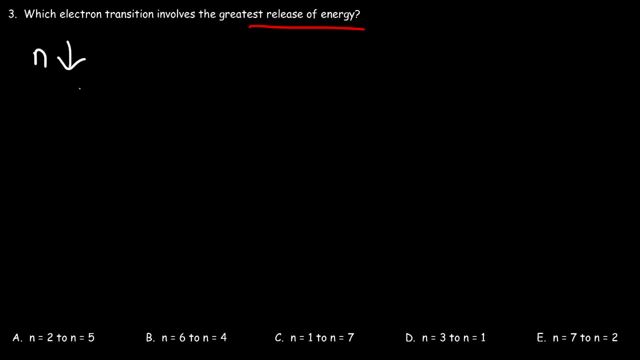 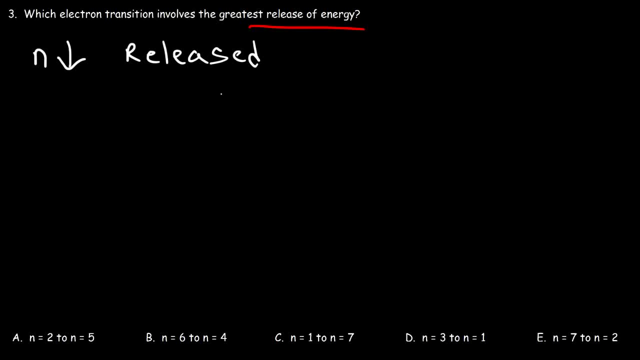 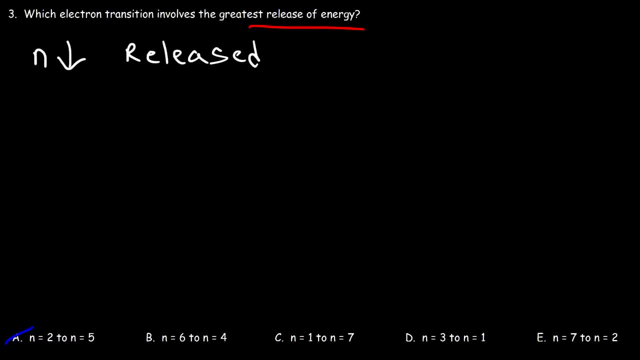 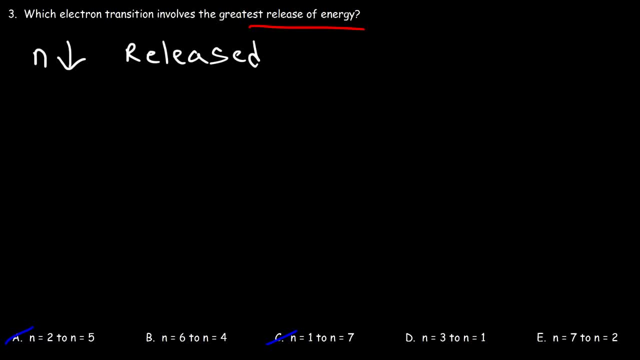 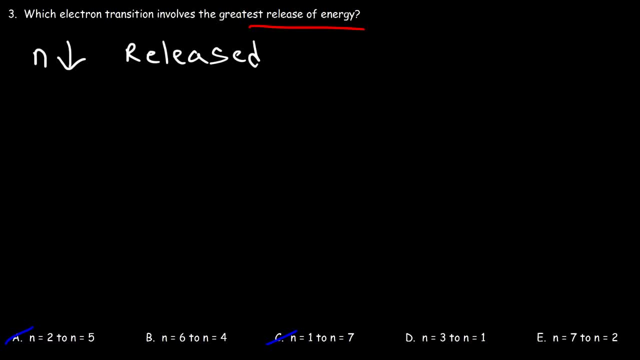 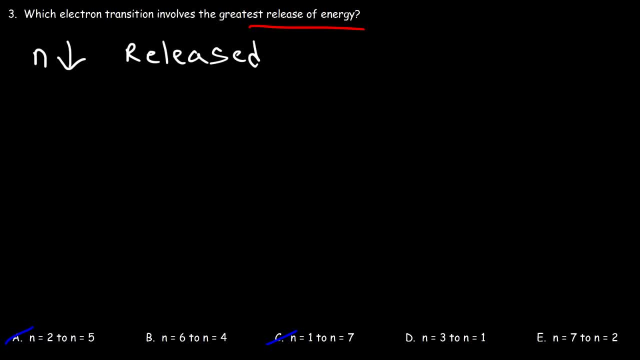 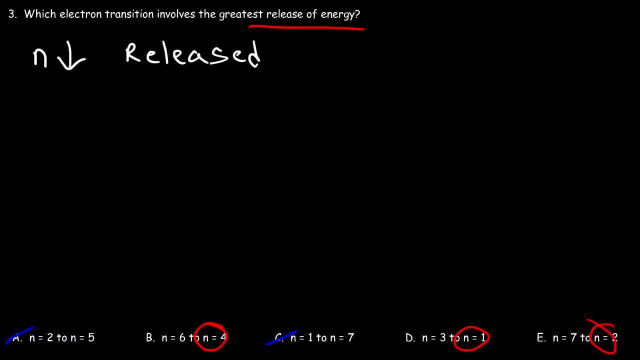 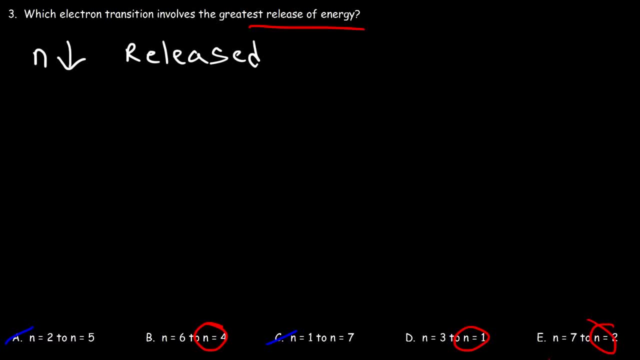 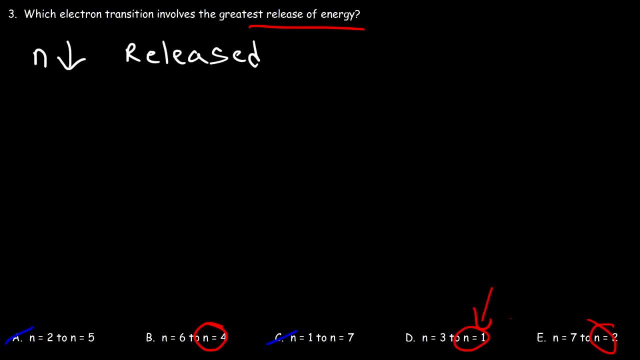 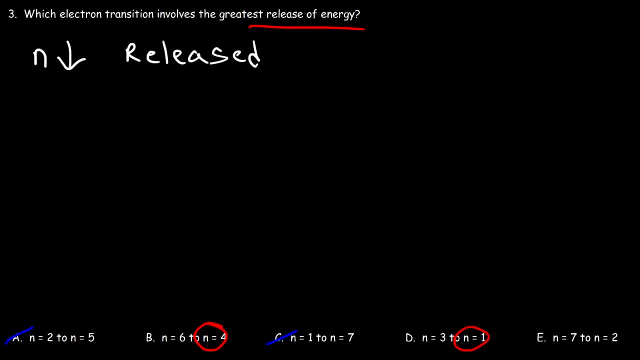 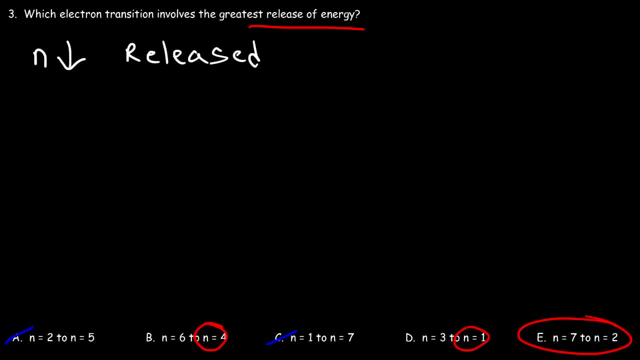 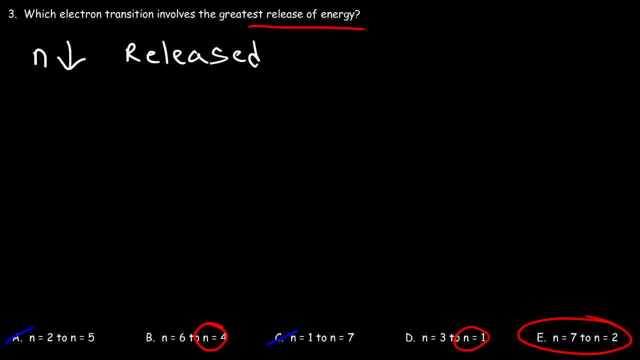 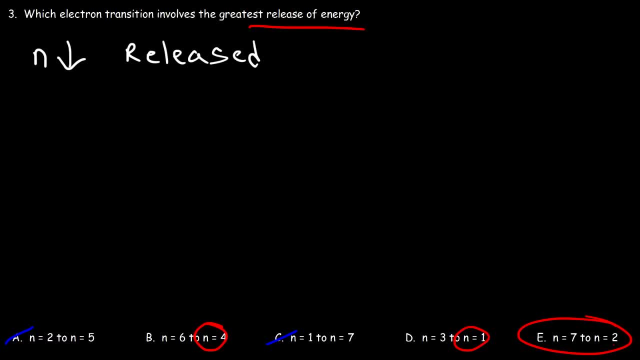 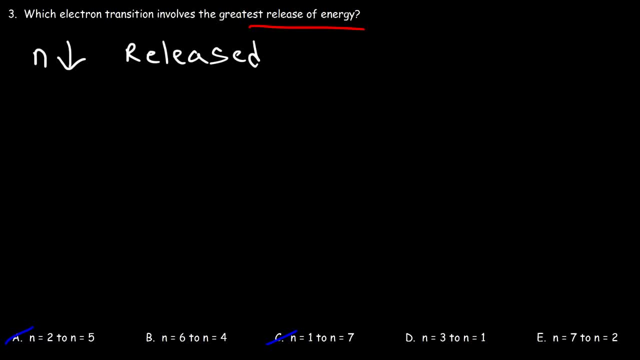 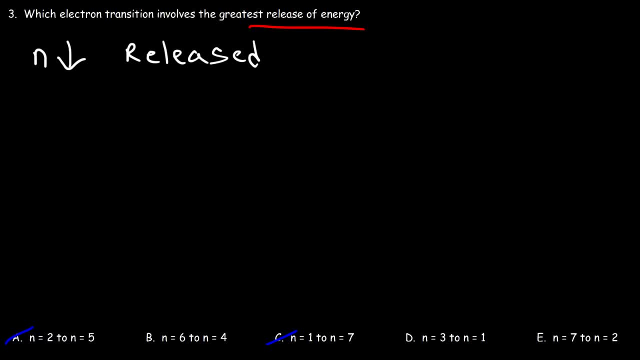 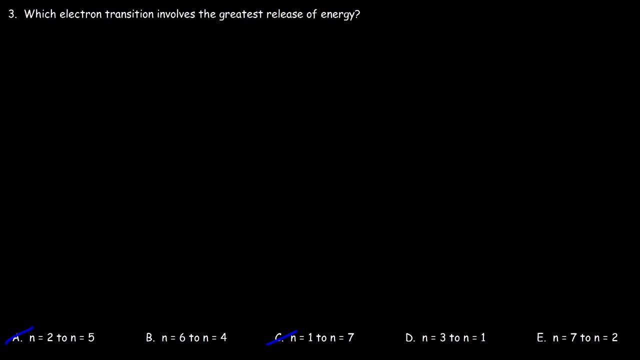 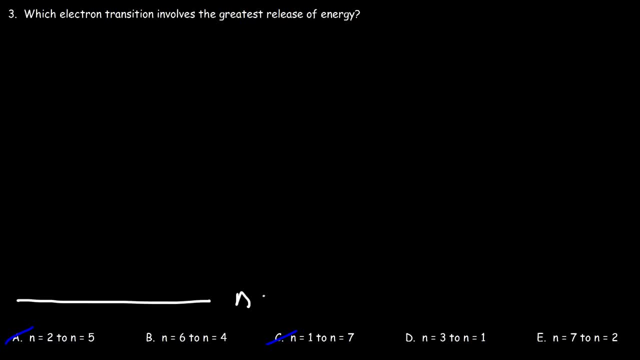 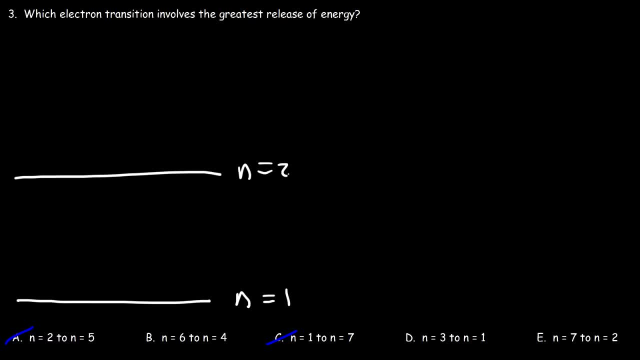 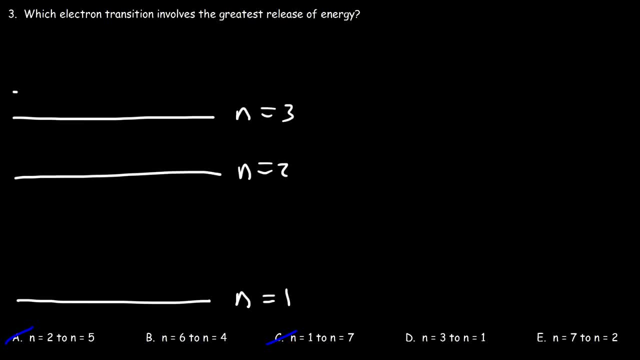 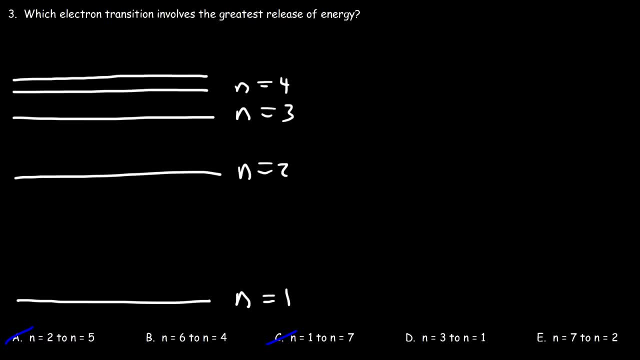 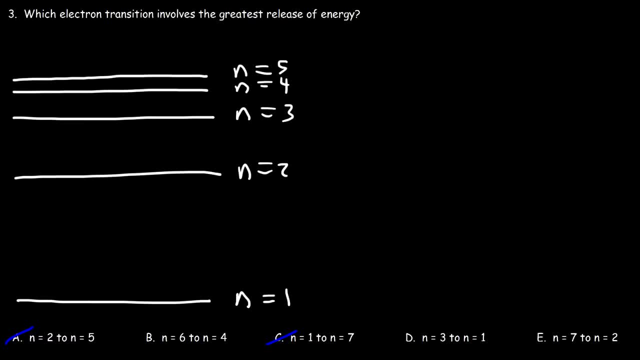 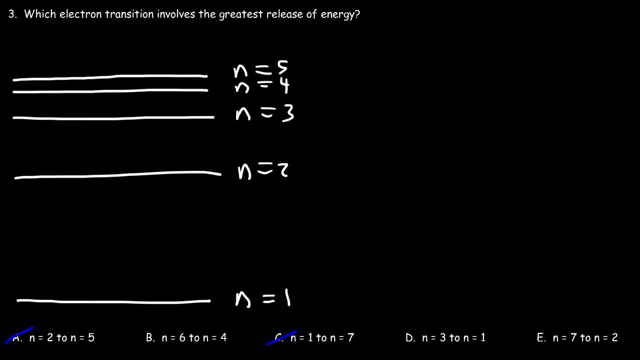 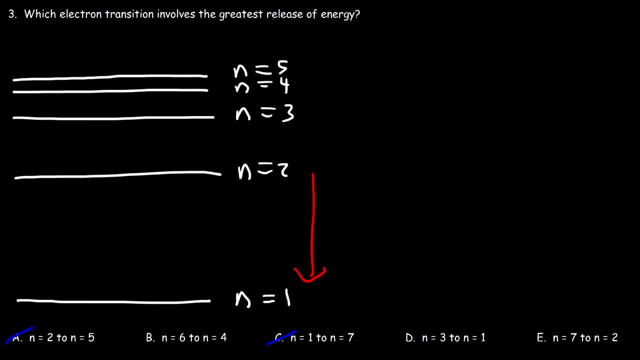 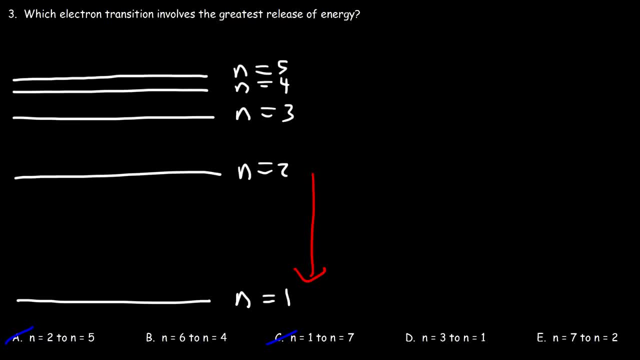 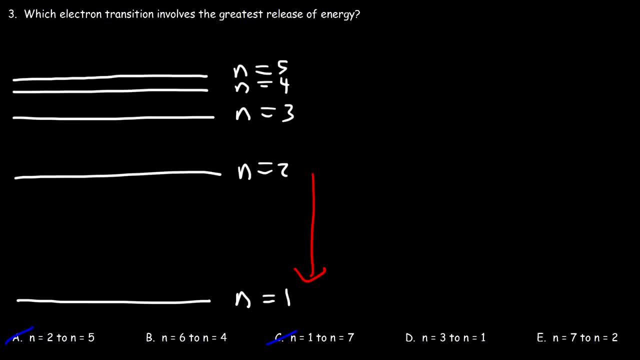 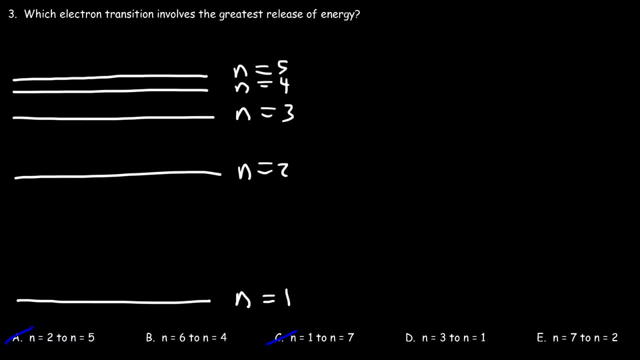 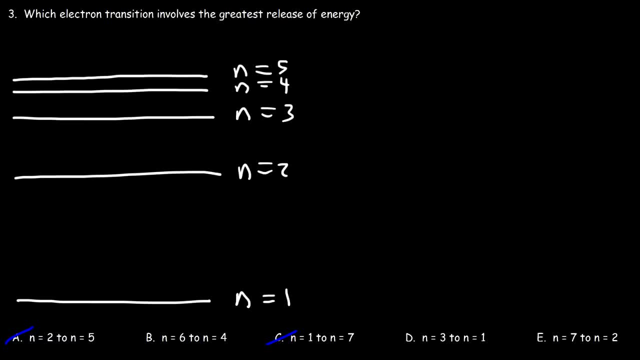 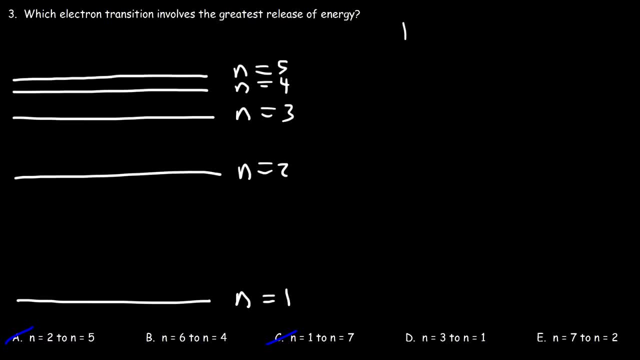 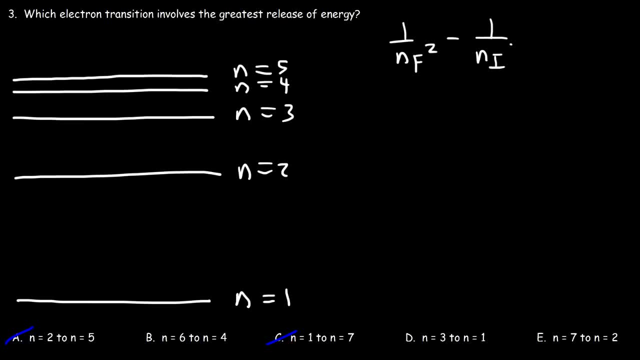 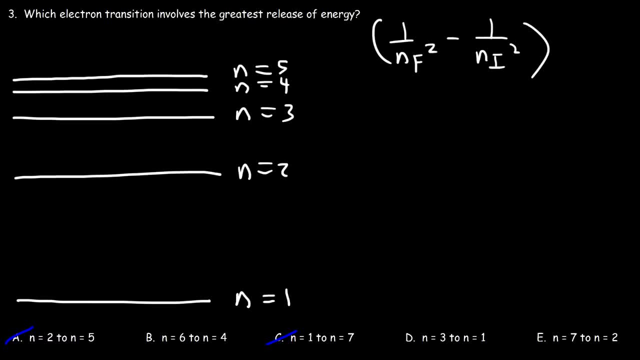 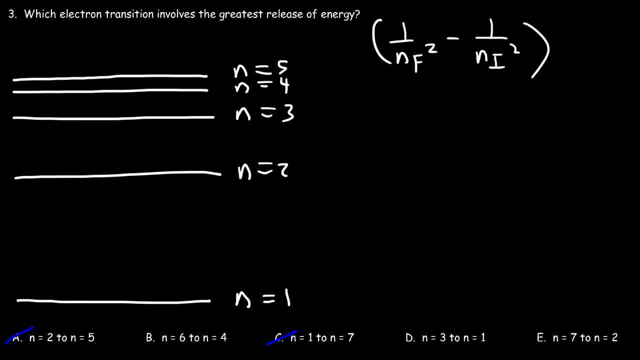 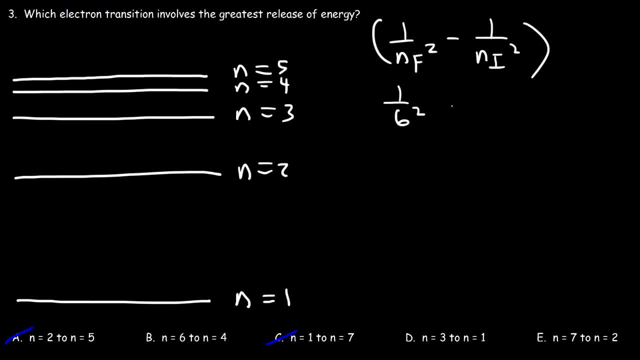 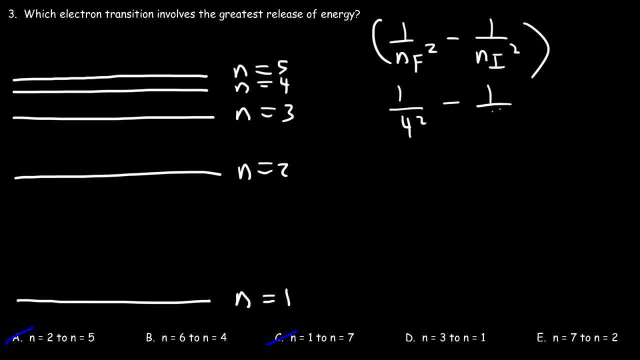 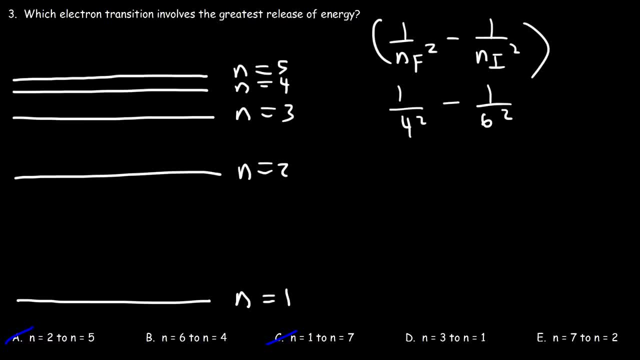 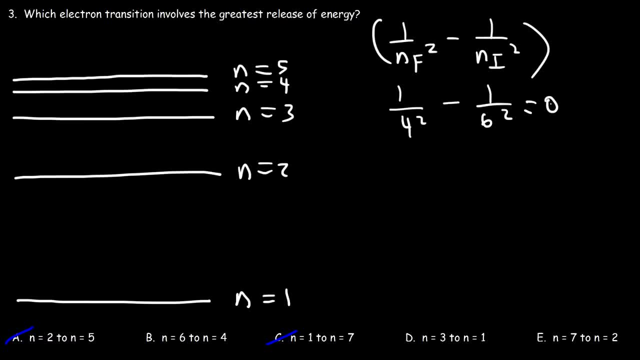 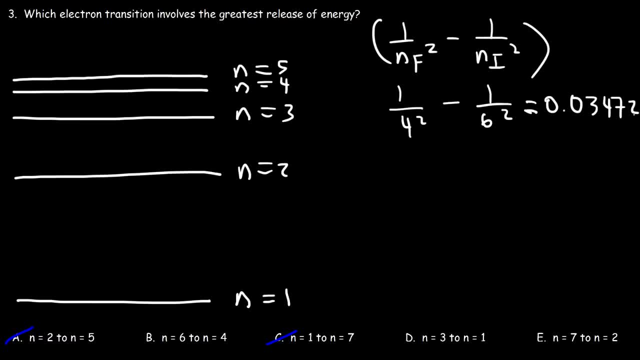 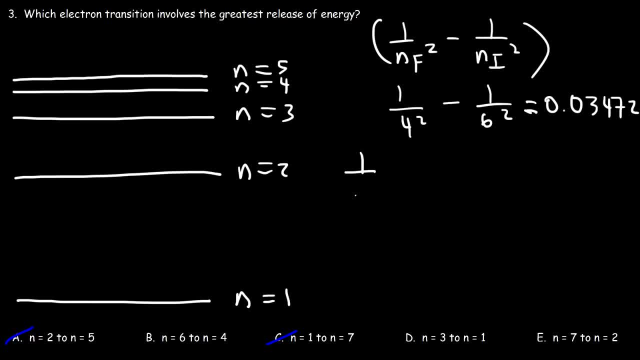 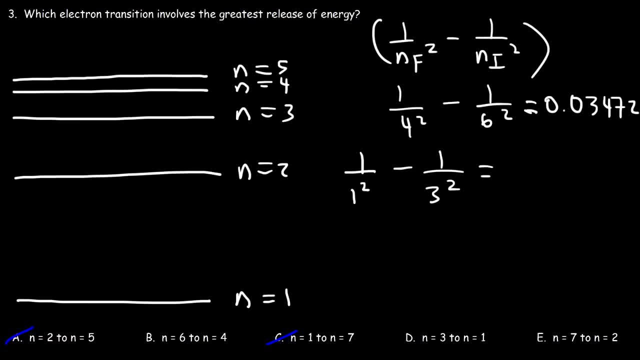 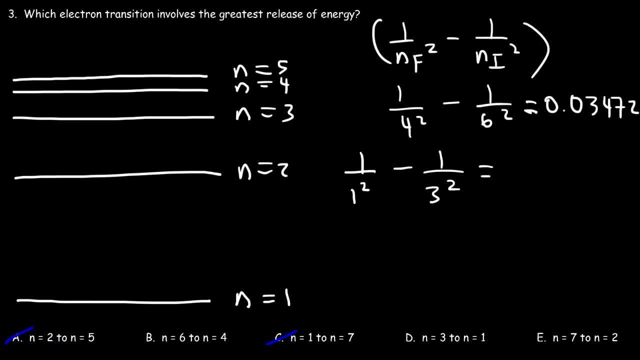 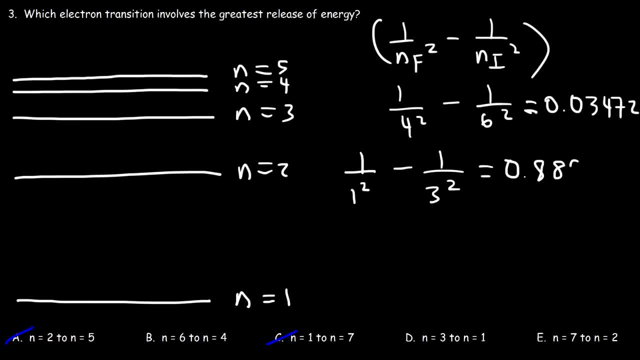 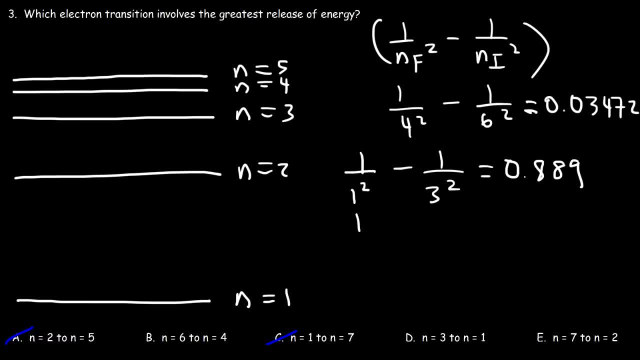 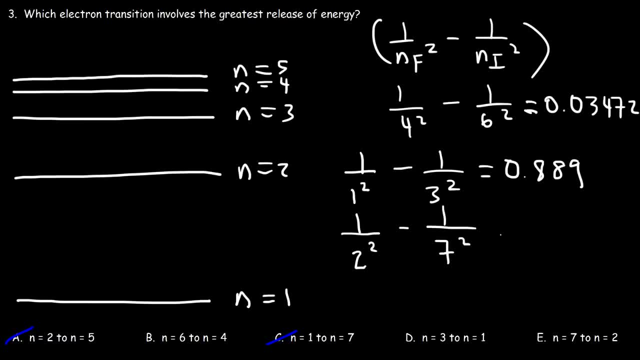 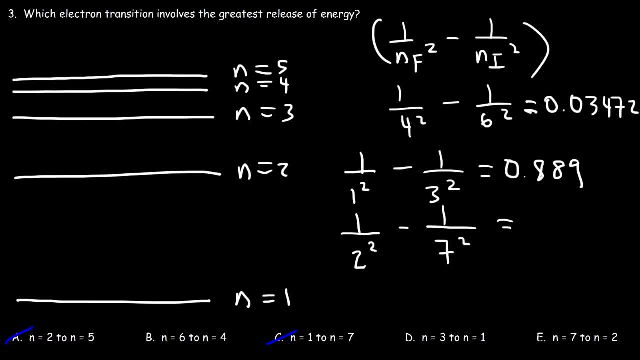 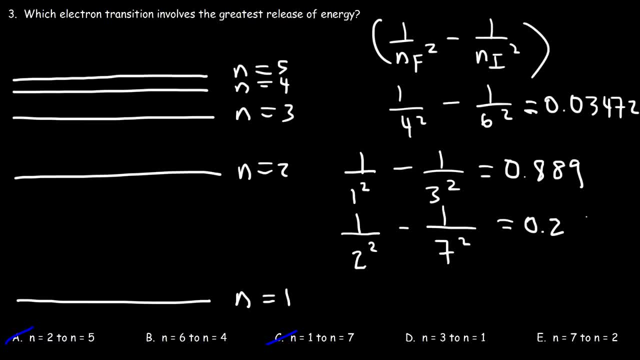 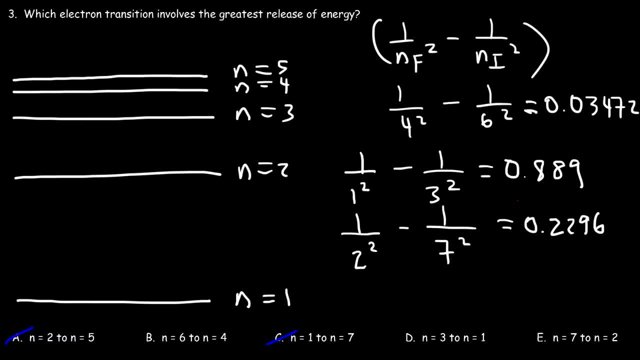 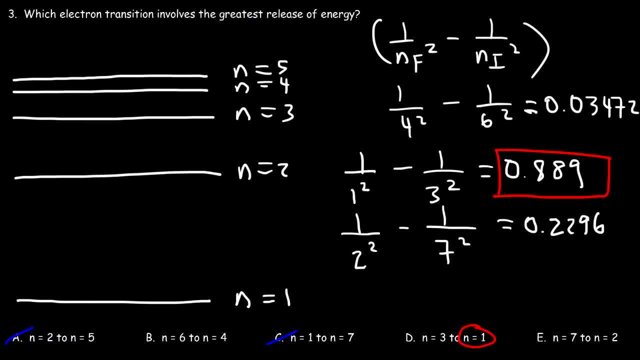 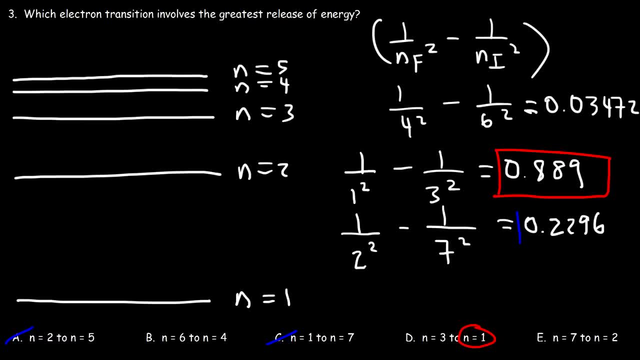 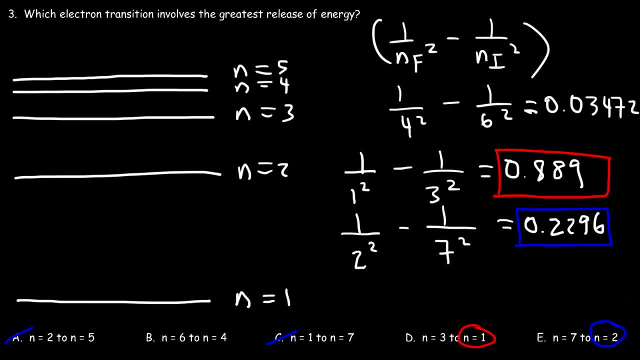 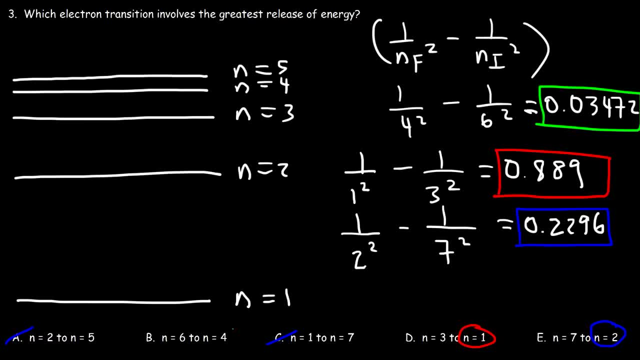 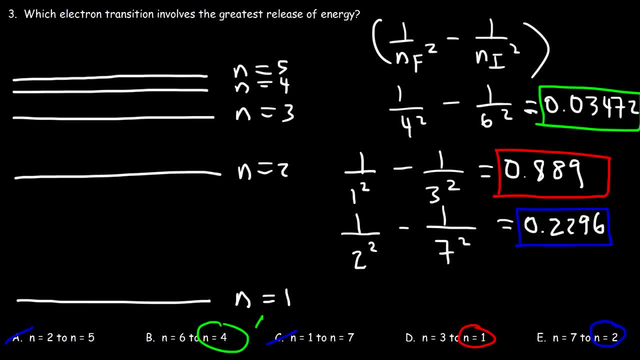 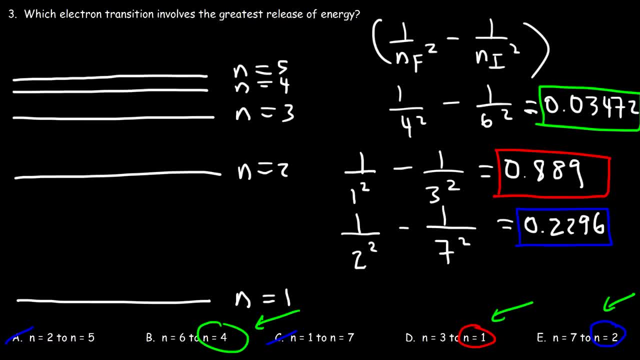 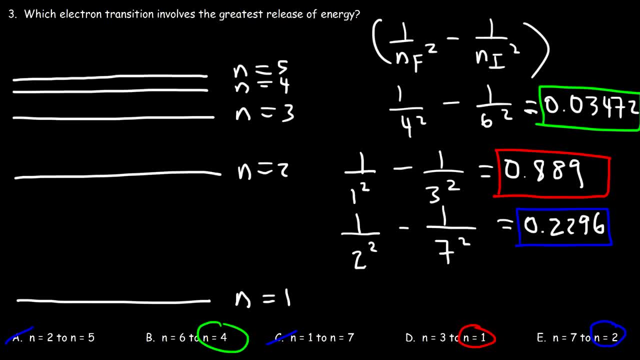 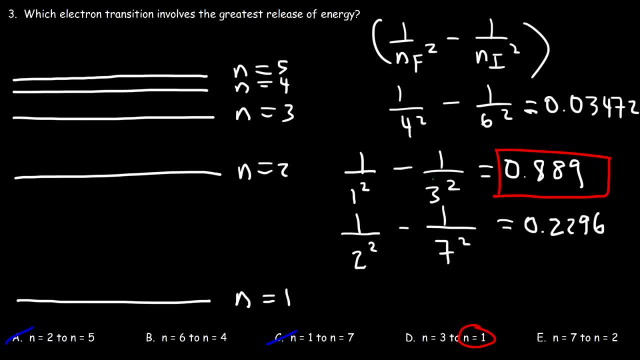 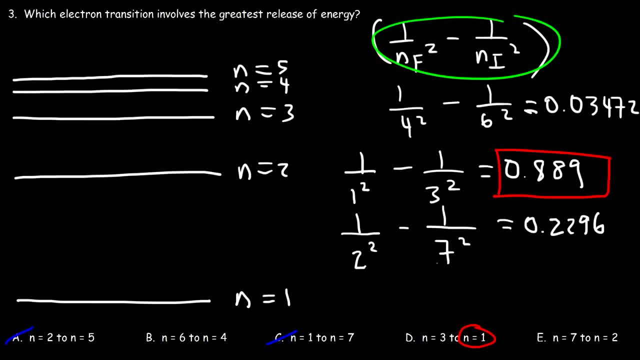 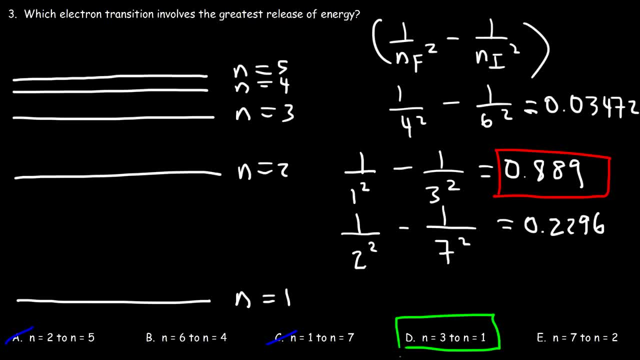 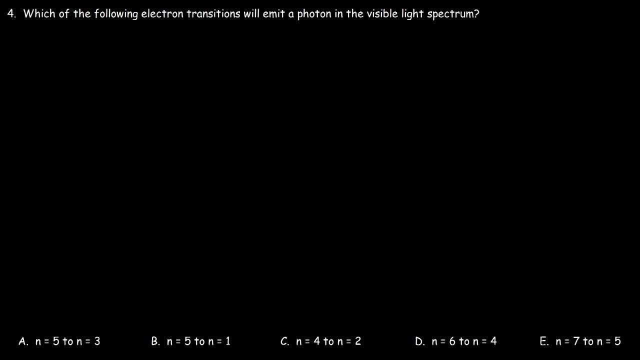 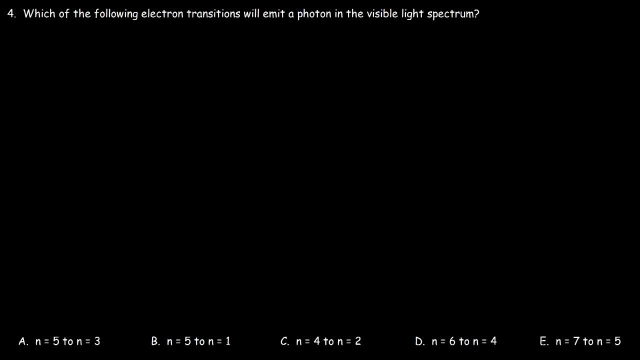 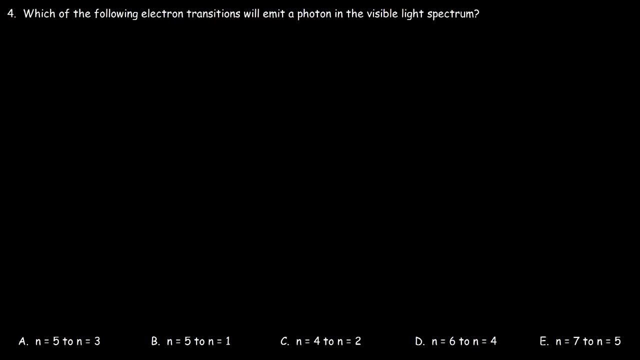 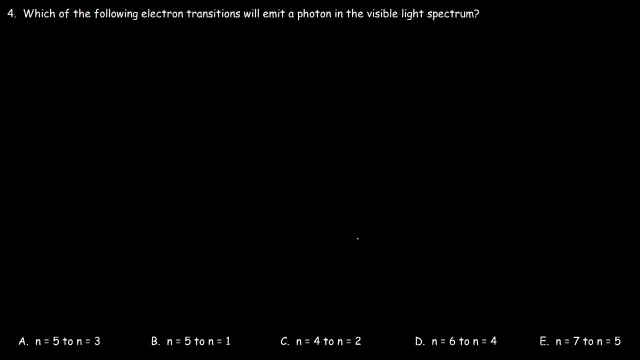 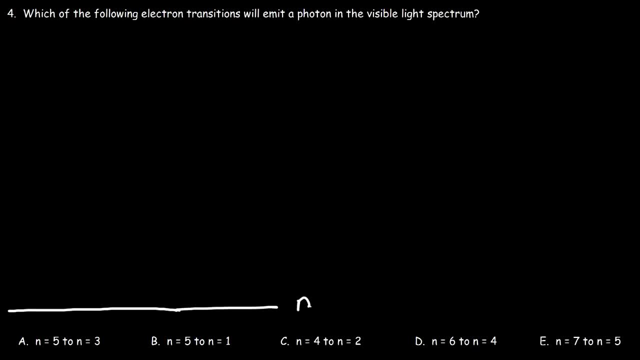 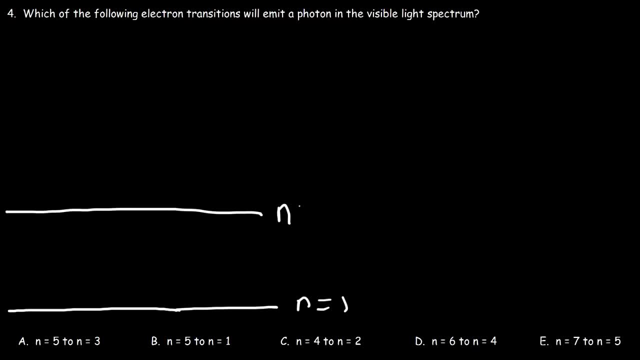 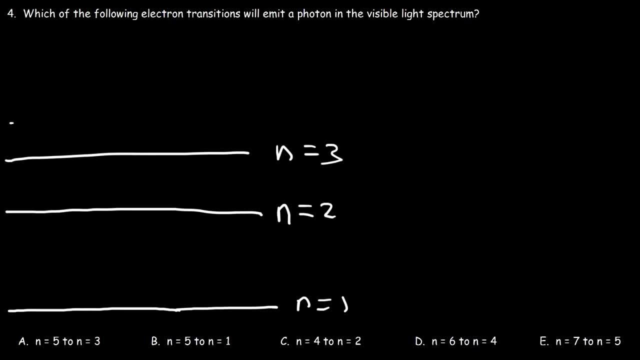 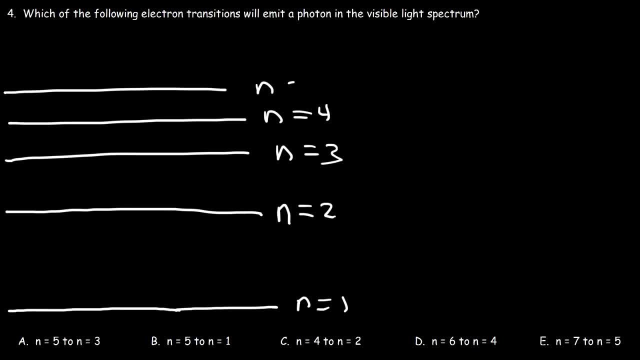 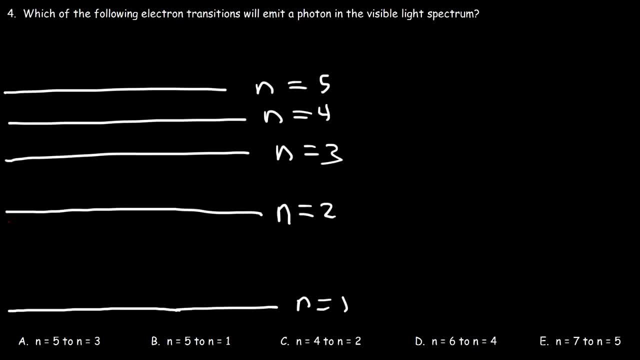 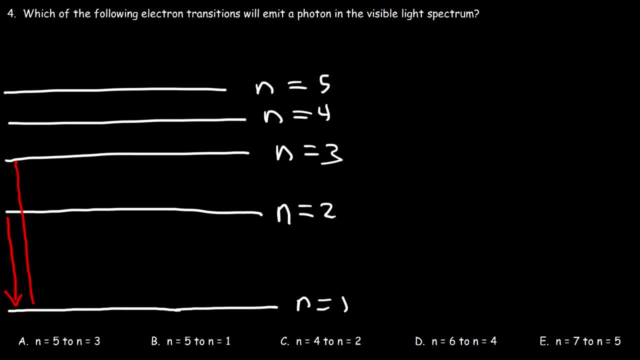 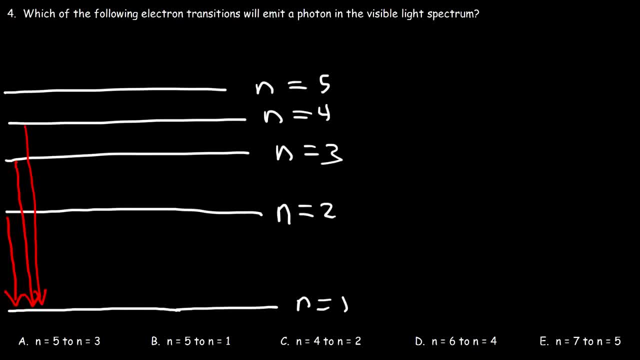 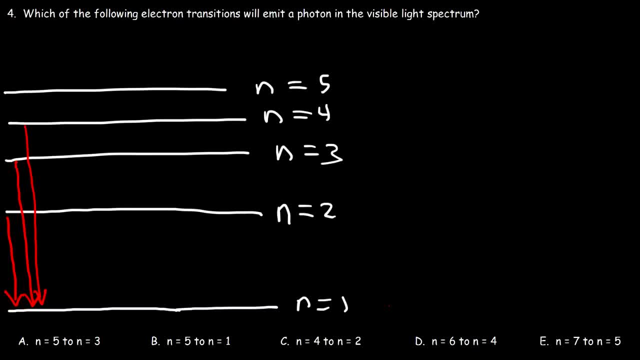 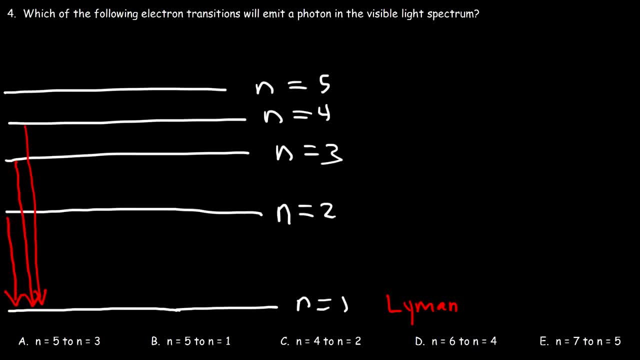 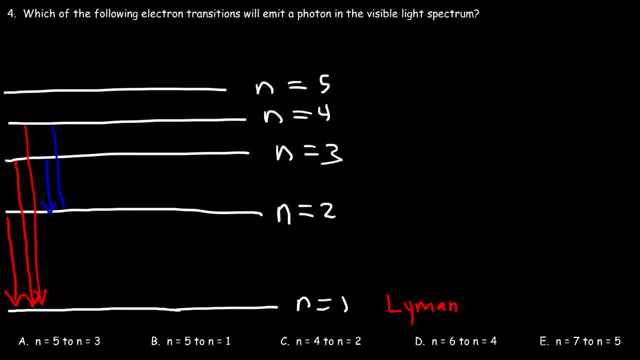 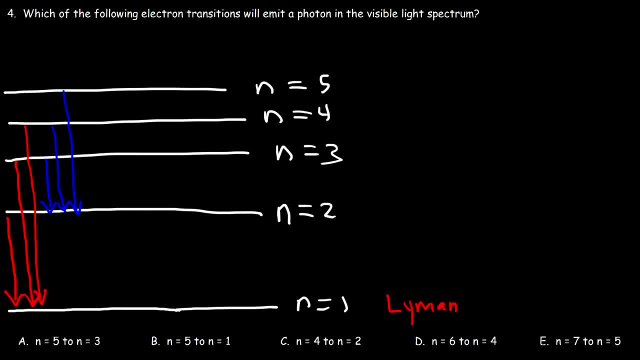 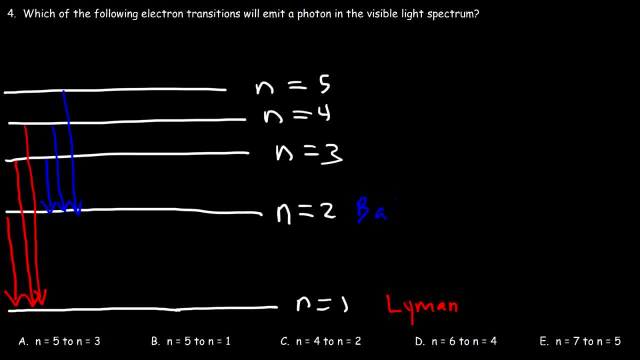 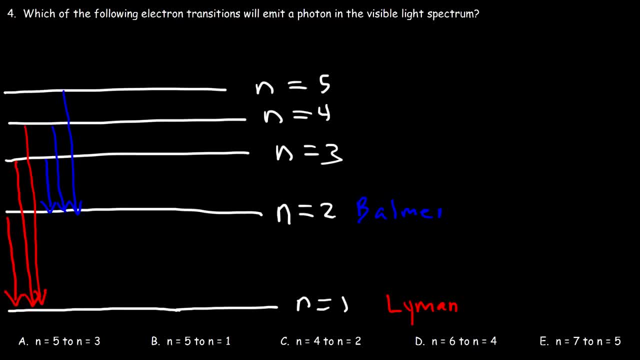 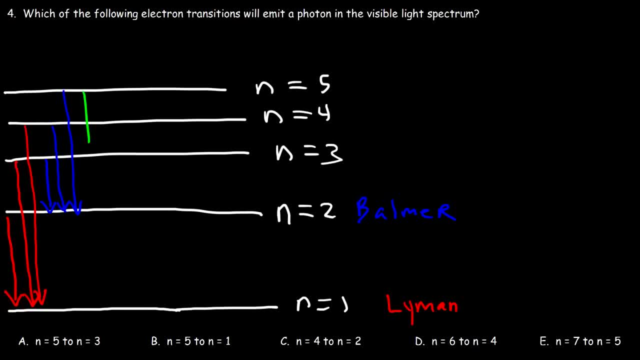 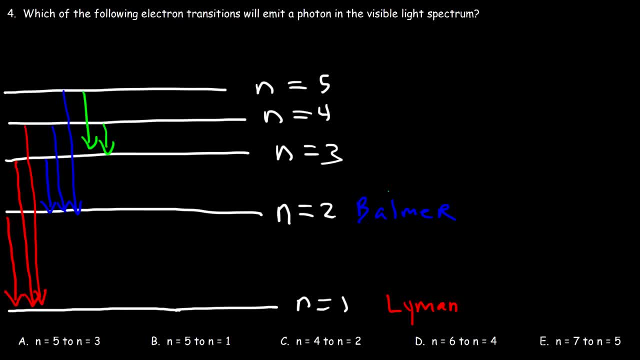 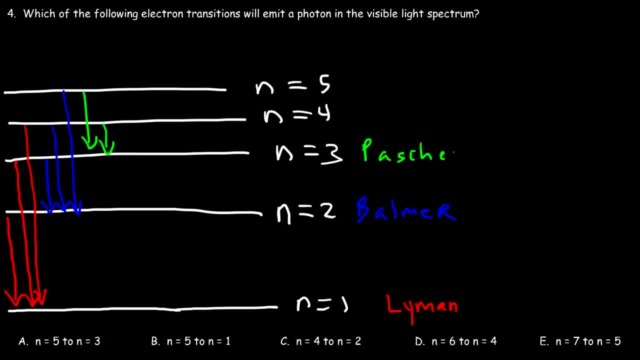 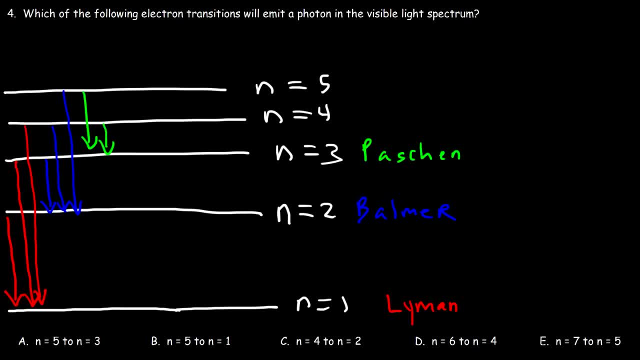 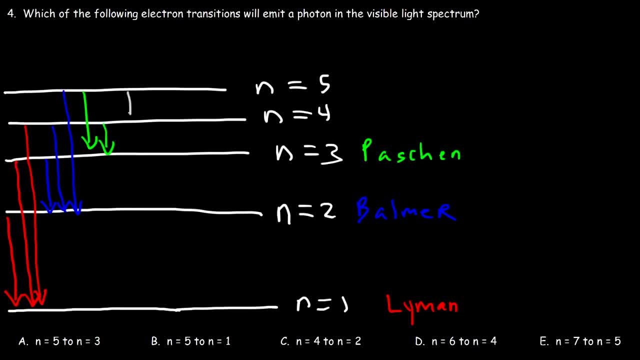 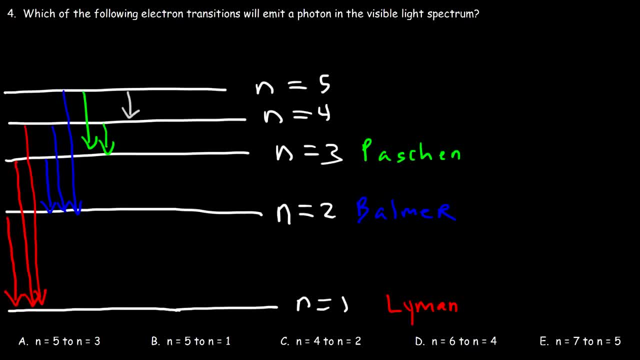 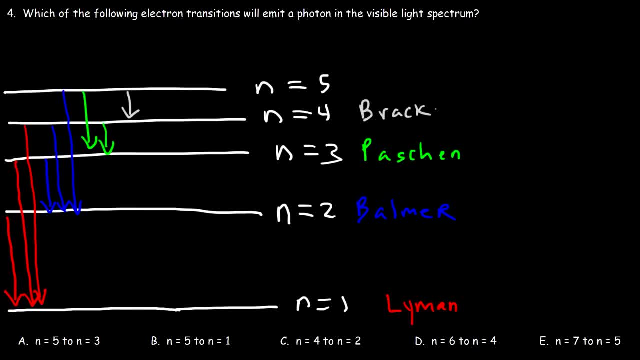 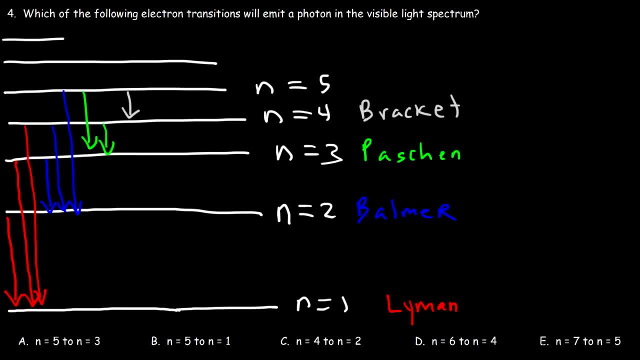 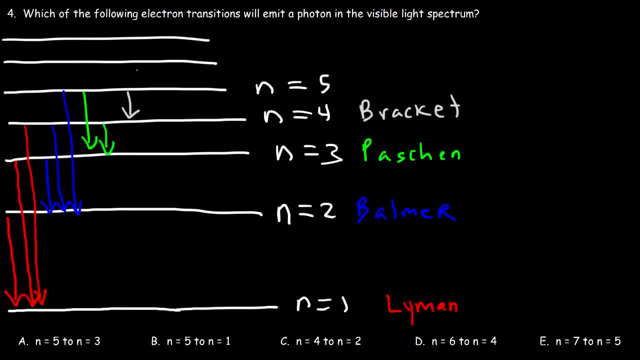 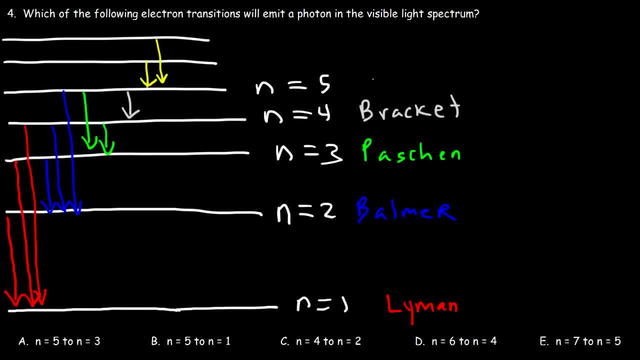 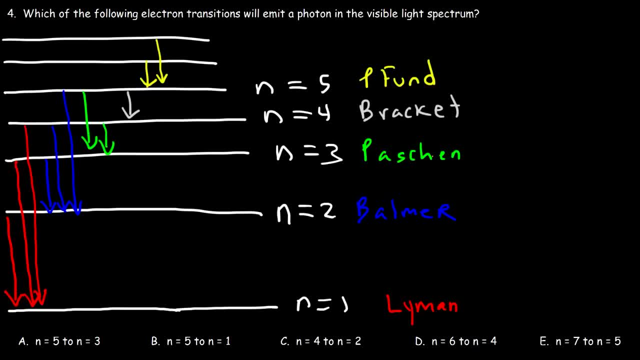 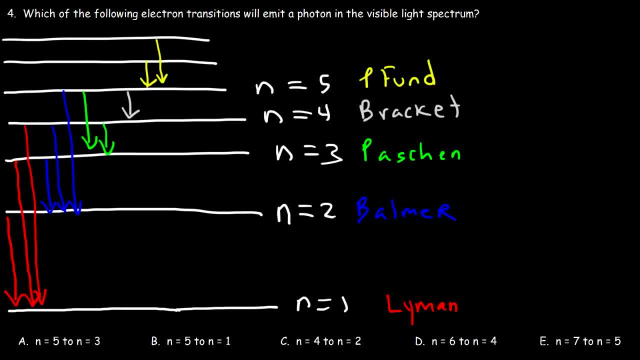 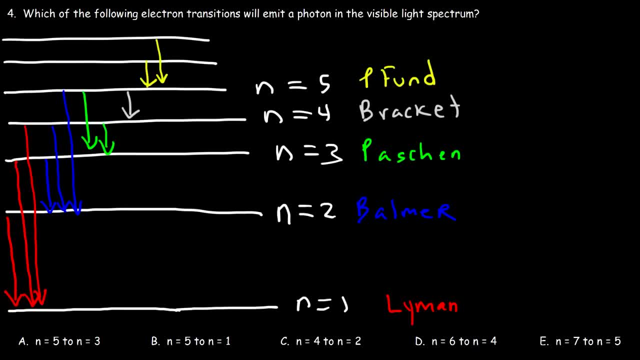 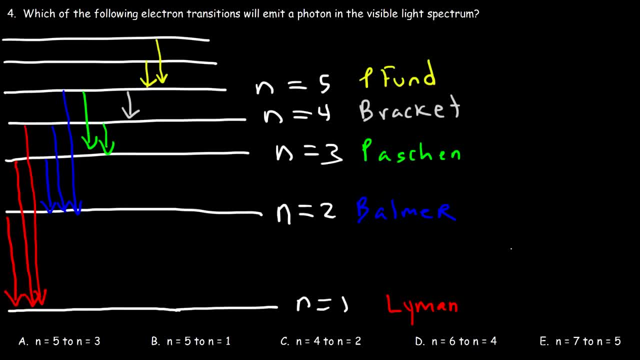 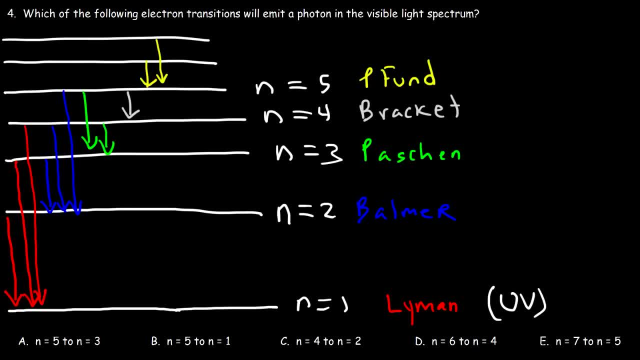 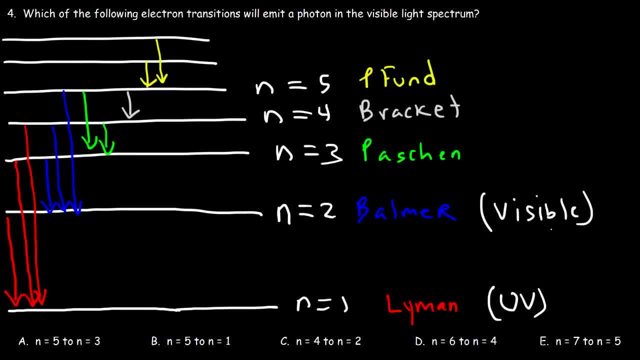 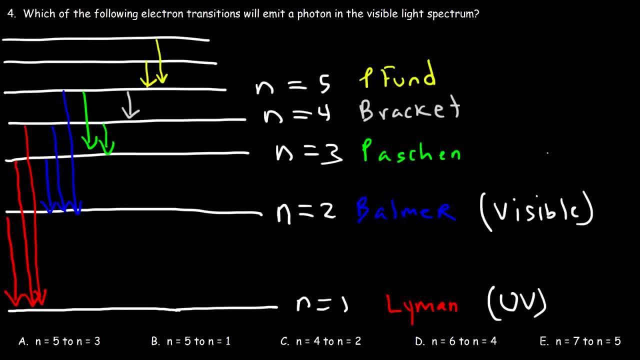 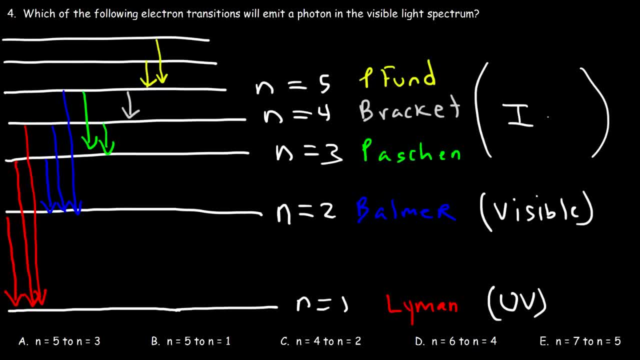 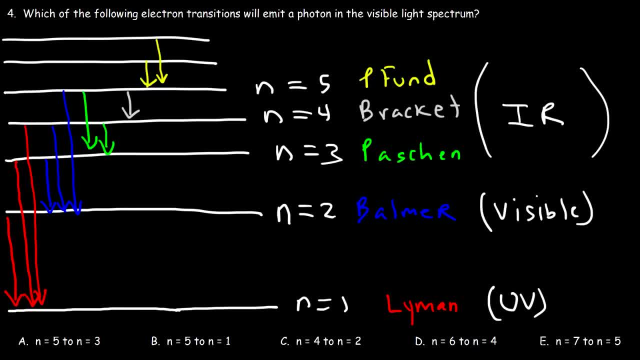 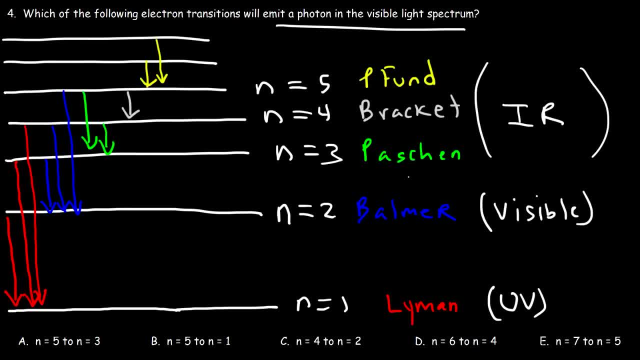 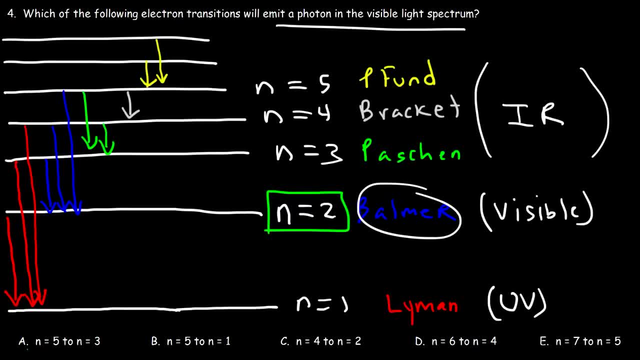 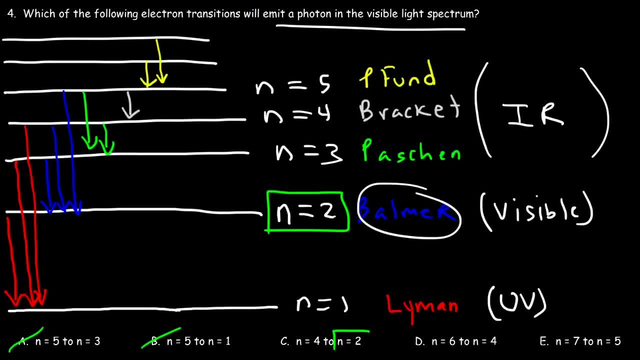 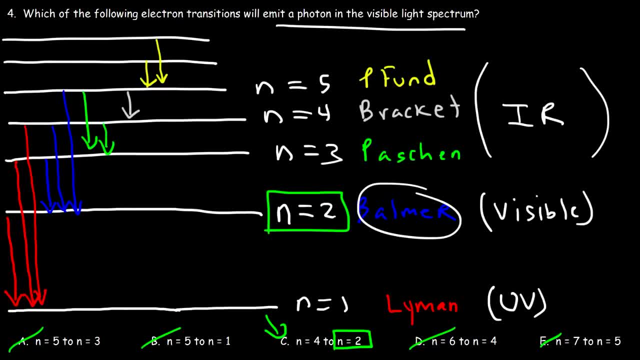 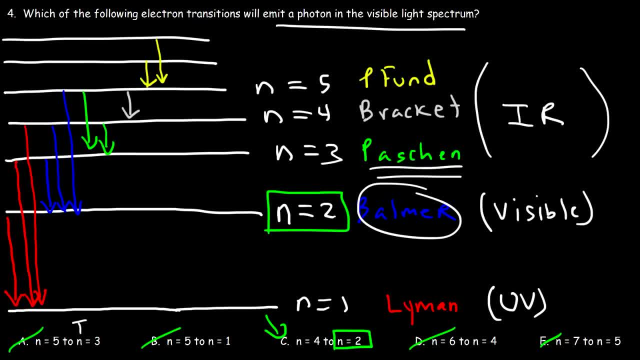 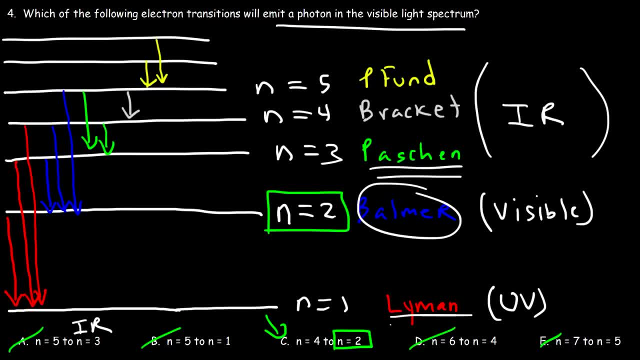 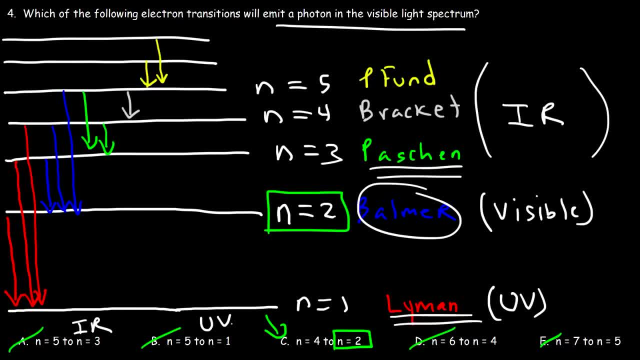 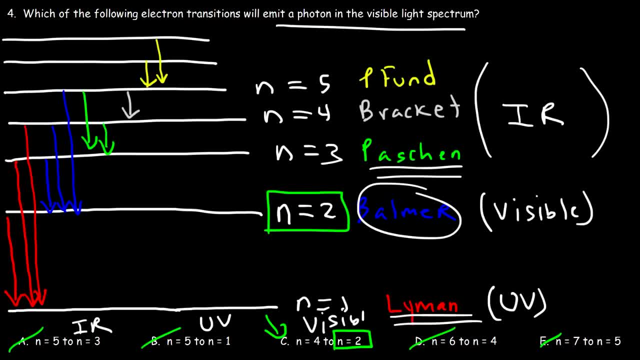 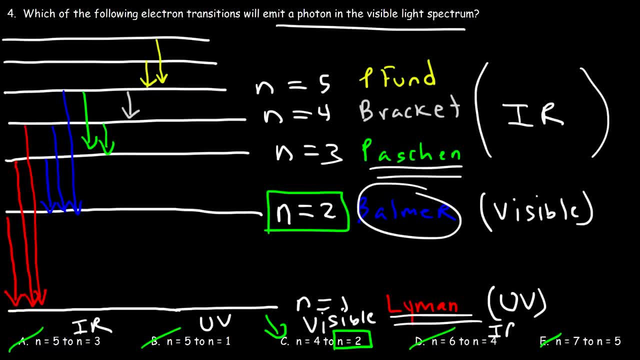 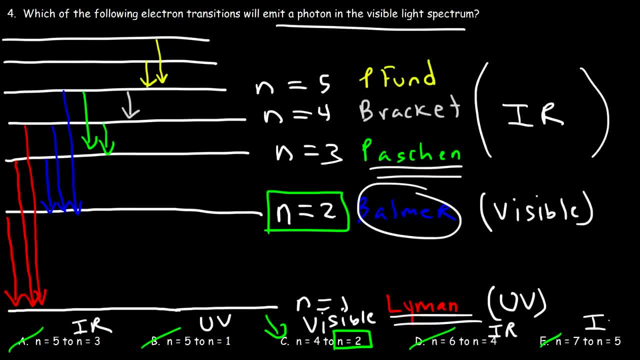 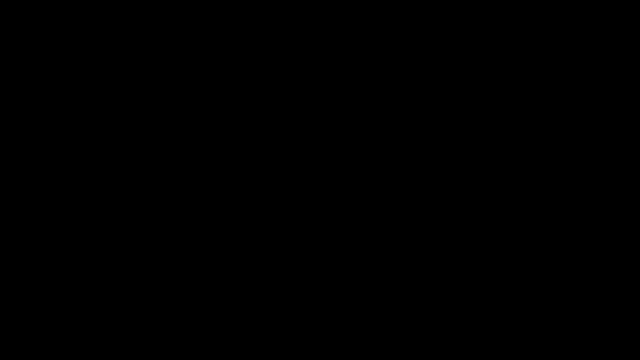 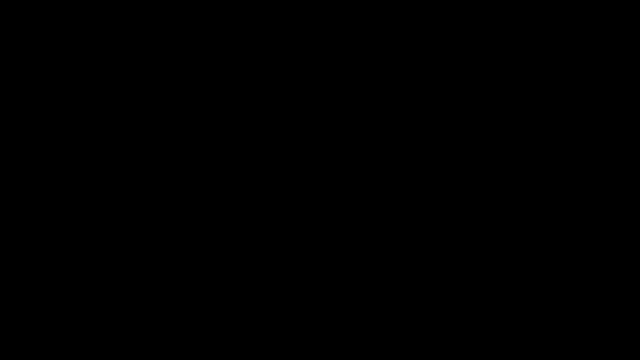 calculate the energy of the photon, So we need to.